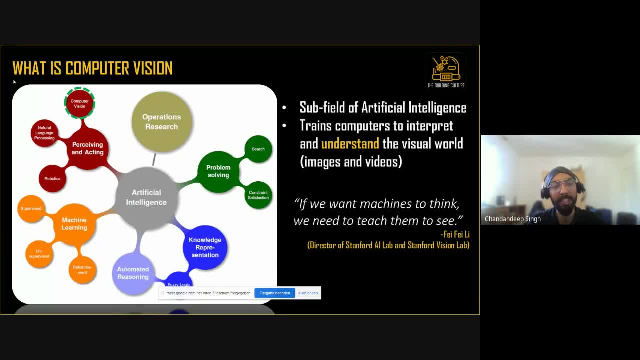 videos And at the same time, we can use machine learning techniques to assist to understand the process, And I'll talk about how that might work in the coming slides. So there's a really good quote by Fei-Fei Li who says that if we want machines to think, we need to teach them how to see. 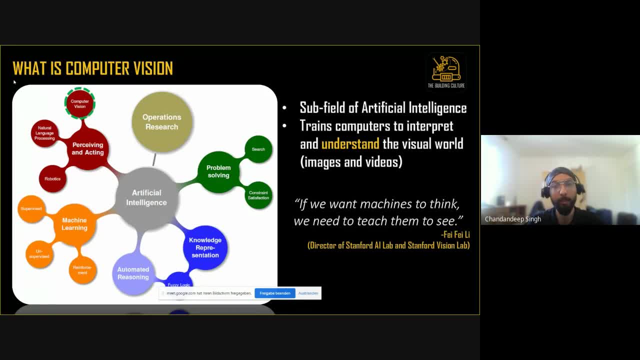 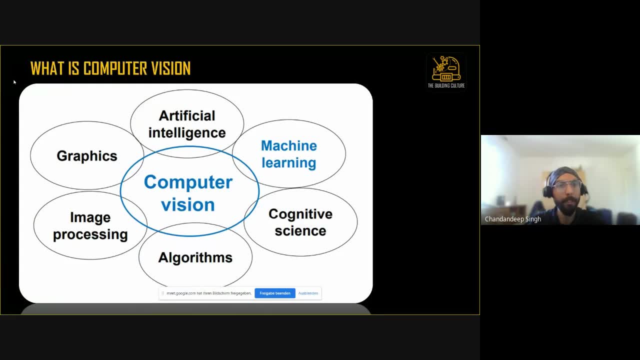 So this is the whole premise behind computer vision. We want to create systems or machines that can learn to perceive and see the environment. So generally, computer vision actually is a very different thing than what we're used to. So what we're used to is that we have to. 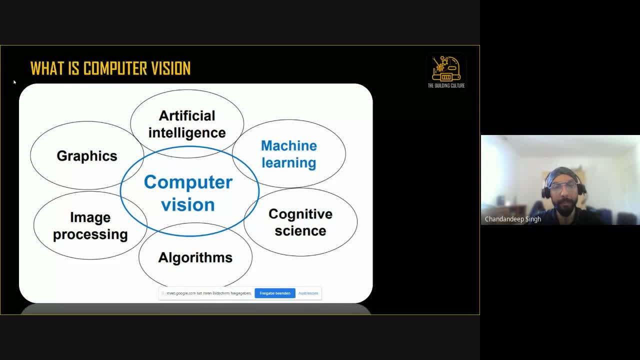 So generally, computer vision actually is a very different thing than what we're used to. So what we're used to is that we have to. It actually consists of a lot of different areas, So it's very interdisciplinary. It has, of course, intersections with machine learning, as I mentioned, and it also intersects with computer graphics, image processing, cognitive science and artificial intelligence, which actually, if you think of the broad picture, artificial intelligence is the broad category and computer vision is the subcategory, but in this diagram it represents it in a different way. 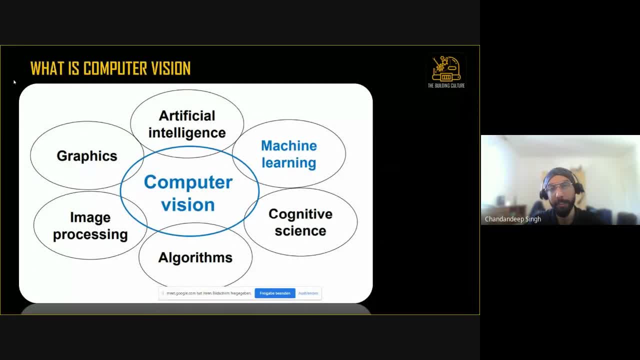 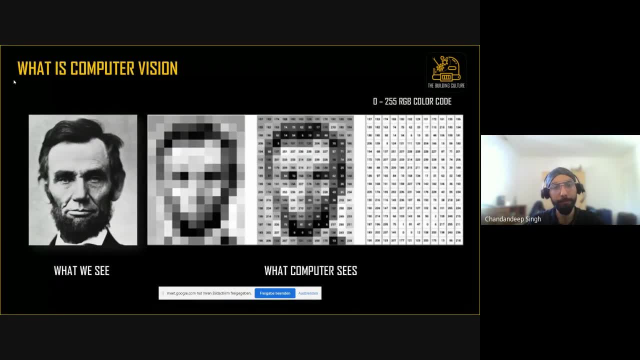 But the main idea that I want to convey is that there are intersections between machine learning and computer vision. So why do we need to learn computer vision? So, for us humans, when we look at a picture, we can perceive that, okay, this is Abraham Lincoln, and we can get to know different features about this, about the appearance of this person. 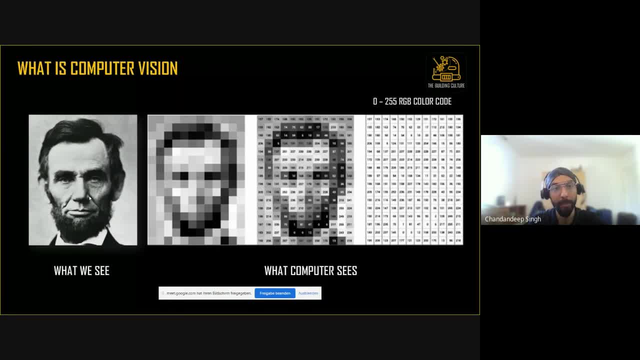 We also have, maybe, emotions attached to the image when we see. We also have emotions attached to the image when we see, So probably link it to our existing set of knowledge. So when we look at an image, we understand it, and this is what we want to enable the machines, the computers, to do as well. 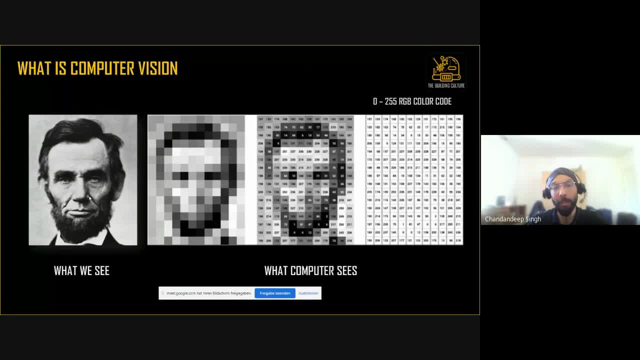 But the problem is that the computers don't inherently understand an image just after seeing it, because a computer works in numbers, as we need to see. So what a computer would actually be seeing it is actually as a computer. So what a computer would actually be seeing it as a computer. 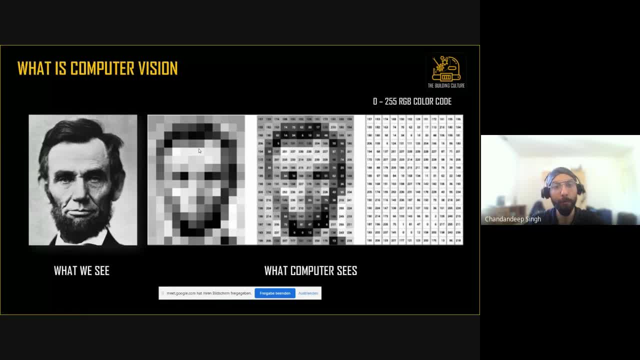 So we have the pixels Now. we have this year as a collection of pixels of different intensities. of course, it depends on the resolution here, but essentially what we would be seeing is a set of numbers Now. So we have the pixels Now. 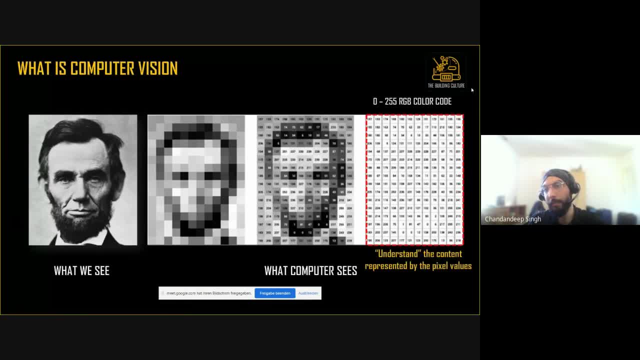 appreciate the complexity of computer vision, You can imagine that if you're just given this set of numbers now you have to make sense of, let's say, what. what sort of numbers would represent? represent the? that's something that's actually more confusing right now. say what, what sort of numbers would represent? represent, let's say, the eyebrows, the hair, the. 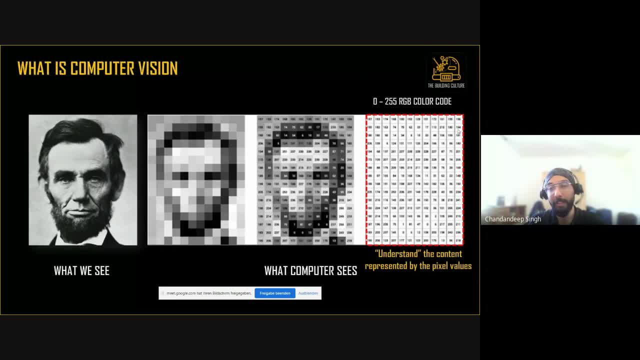 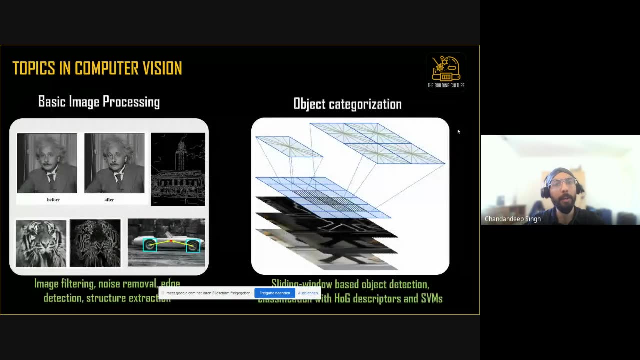 jawline and other features. so it becomes really complicated to teach the computer to understand several aspects of an image or even a video, and this is what we try to do with computer vision now. there are a lot of topics in computer vision actually, and which is also the reason why it is. 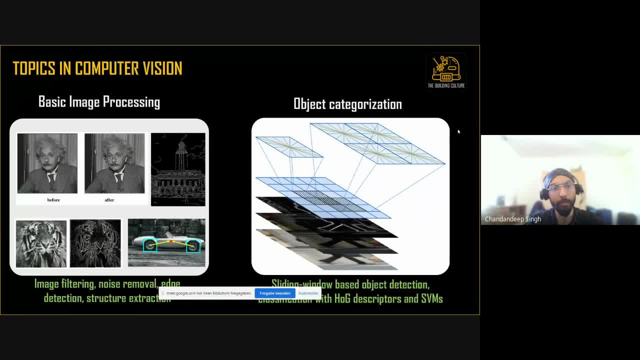 a bit challenging to start learning computer vision. so one of the key things is basic image processing- that that is actually a part of computer vision. some people can say that it's a different field, but there are intersections with it. so, regardless of how you view it, a basic 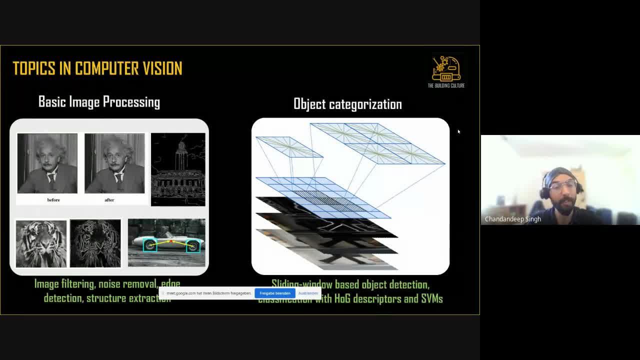 basic image processing is essential to start learning computer vision and what we mean by basic image processing. when we talk about image processing, we talk about filtering images- you know sharpening these images, these basic instagram filters, for example. you you talk about identification of edges, noise removal, structure extraction- you know extraction of blobs or circles in images and so on. 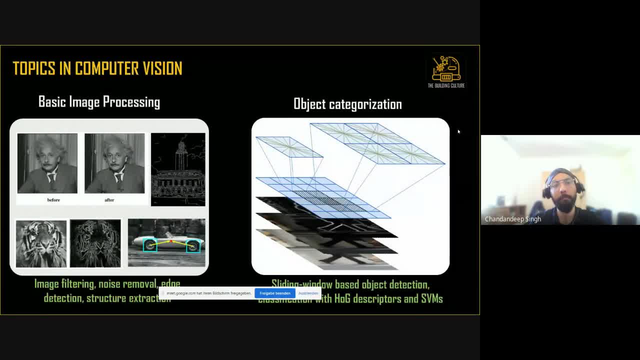 so these fall under the category of computer vision. the reason why this is important is because, even if you use neural networks- uh you know, for your computer vision problem- essentially you would have to do some sort of pre-processing to make the images or the data set suitable for the machine learning. 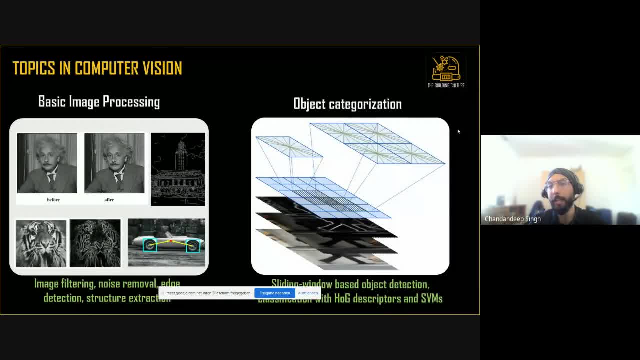 or the neural network model being used. and then another category is that of object categorization, and here we use, let's say, a sliding window based object detection. we use classification with the hog feature descriptors and support vector machines. so these essentially talk about using a conventional machine learning approaches or even conventional 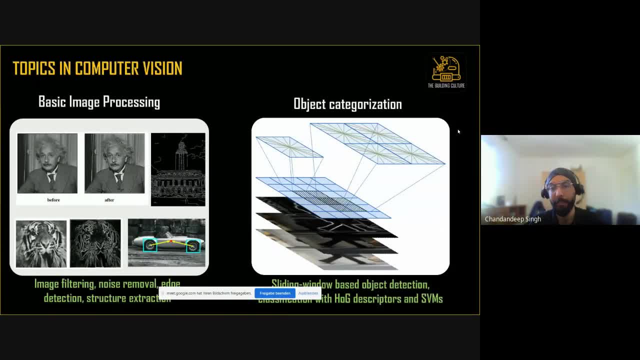 computer vision approaches for performing object categorization. so the image that you see here is that of hog descriptors. i'll not go into details of all of these specific approaches, but the point would be that i give an overview of all the approaches and how you can actually start learning. so 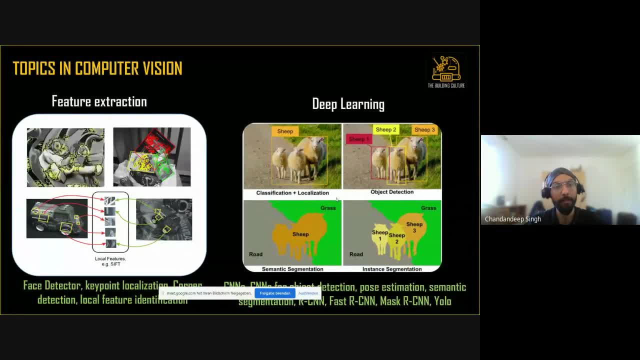 another thing you might have heard is that of feature extraction. now this is when we talk about feature extraction. we are talking about manual feature extraction using conventional computer vision approaches: face detection, key point localization, corner detection, harris corner detectors, local feature extractions, extractors like sift surf etc. come into play and then 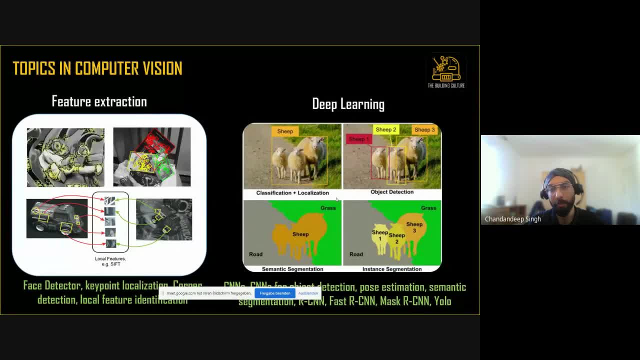 deep learning also assists in computer vision. so the nowadays this is when people talk about computer vision, this is what they talk about actually. but there are a bunch of different aspects of computer vision, as we saw as well. so we see here that classification and localization of objects inside an image, 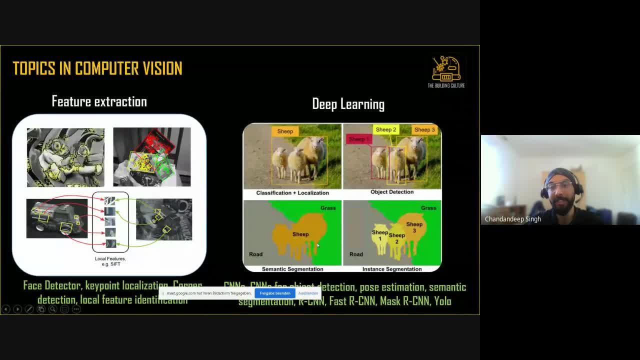 identification and detection of multiple objects inside an image. semantic segmentation, which you see here, is we are not separating the individual objects- or sheep in this case- but rather having a have a general sort of segmentation of different types of objects and then instant segmentation. so all of these things are more complicated tasks and 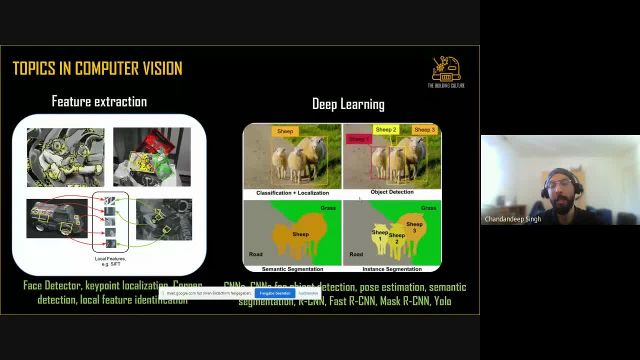 that is why deep learning assists in these tasks. so this is where convolutional neural networks come into play, and also these are also used for pose estimation. so when you have seen these videos where the pose of a human is visible as well, semantic segmentation, ask: mask rcn and fast rcn and yolo. 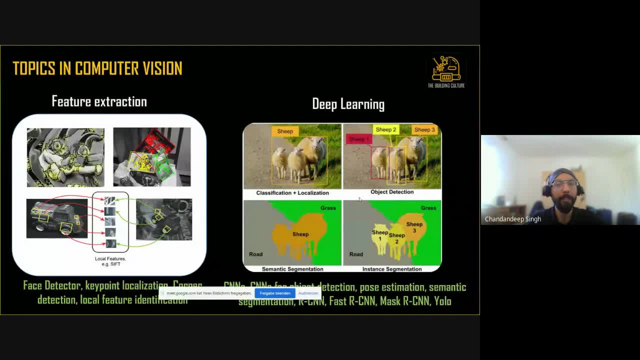 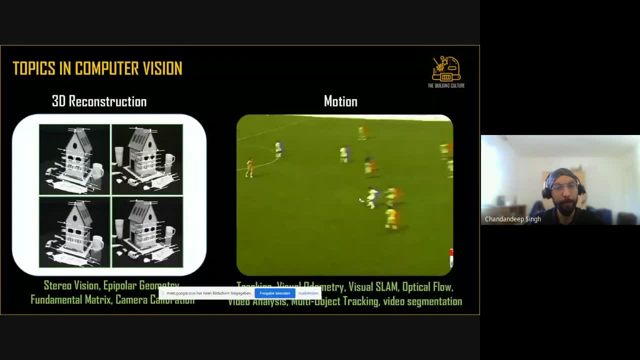 all these kinds of models resonates. these fall under the category of deep learning. but there are also more advanced topics in computer vision, that of using a stereo camera to actually perform 3d reconstruction, and these use concepts like essential and fundamental matrix epipolar geometry. also camera calibration and triangulation approaches would fall under these categories. 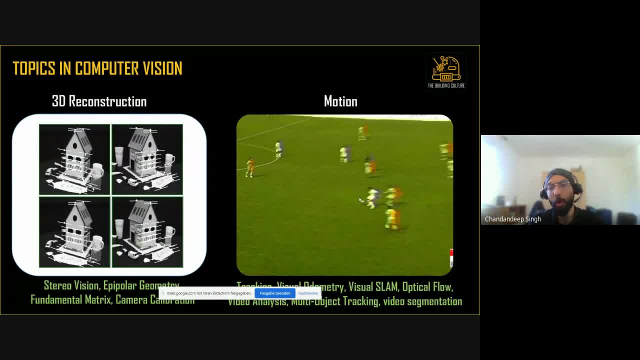 and then after that we can move to talk about motion and talking about how segmentation approaches and 3d reconstruction approaches can be done for videos. so we talk about tracking, template tracking and other lucas canada tracking approaches that are used, and then visual odometry, visual slam, optical flow, video analysis, multi-object tracking and video. 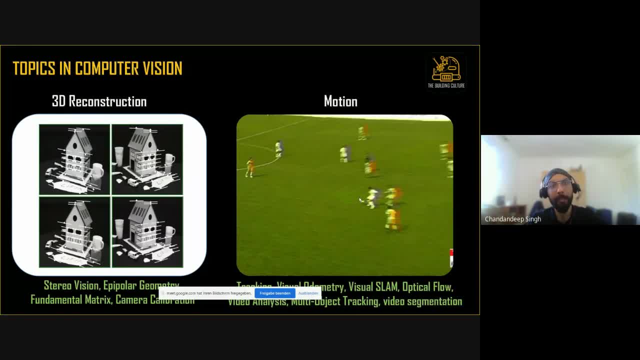 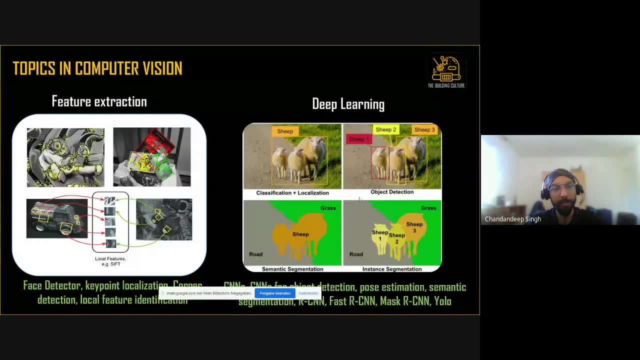 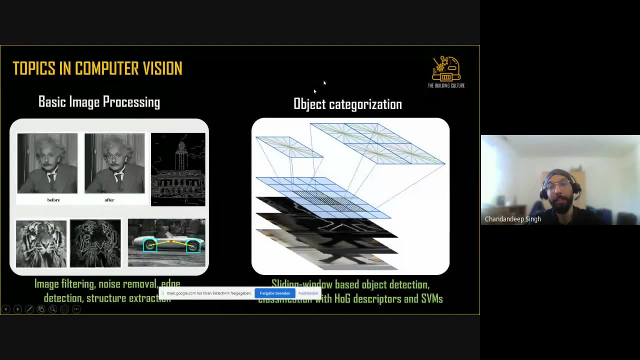 segmentation. so all of these seem like a lot of things to learn, right. that is why it's a bit tricky to get started with computer vision. so the idea is that you start with learning basic image processing and then you learn conventional object categorization approaches and then you move on to learn feature extraction and then 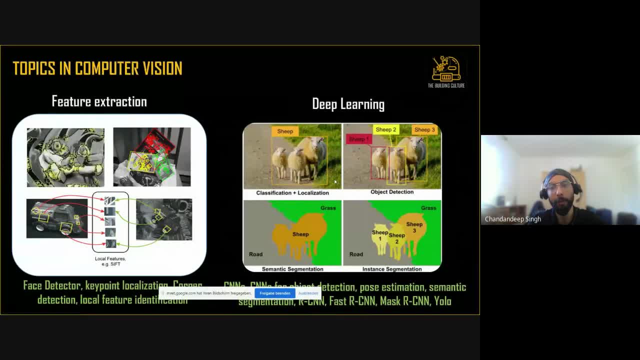 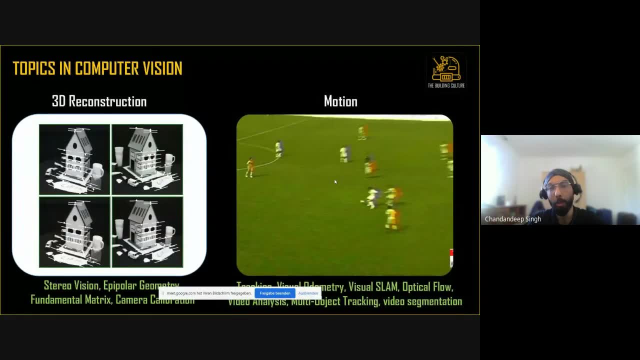 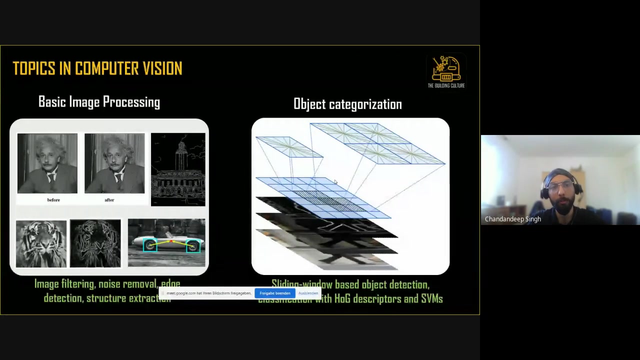 deep learning, which essentially automates the process of feature extraction. then you can go on to 3d reconstruction and then go on to more motion driven approaches. so this summarizes all of the different approaches that are existing in computer vision. now the the, the typical university courses, let's say, would follow to a certain extent. more or less they. 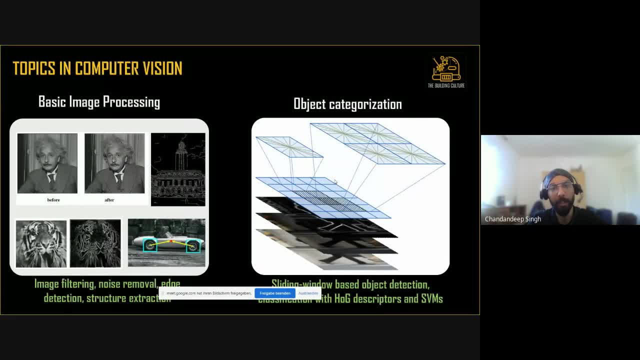 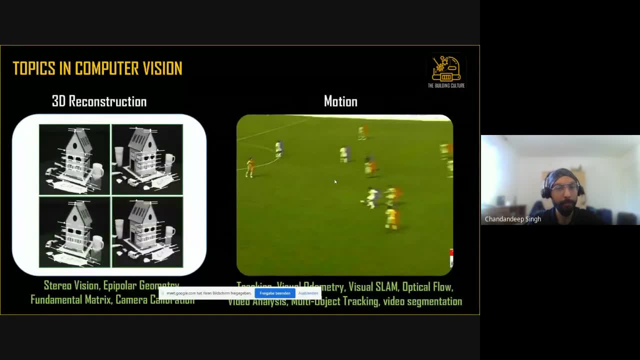 would follow a structured approach where they would start sequentially from basic image processing and go on to, let's say, motion and video analysis approaches. but but my personal experience has been that this is not the best way to learn. first of all because you would be learning lots of theory. 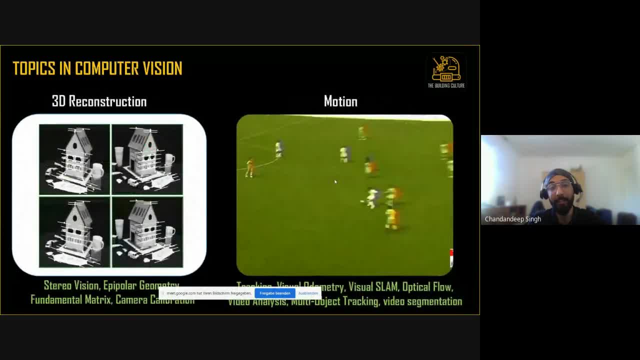 in all of these areas and of course you would be learning lots of theory in all of these areas and of course it's very difficult or next to impossible to do projects in all of these areas. so my view is that you first identify what areas you are interested in. 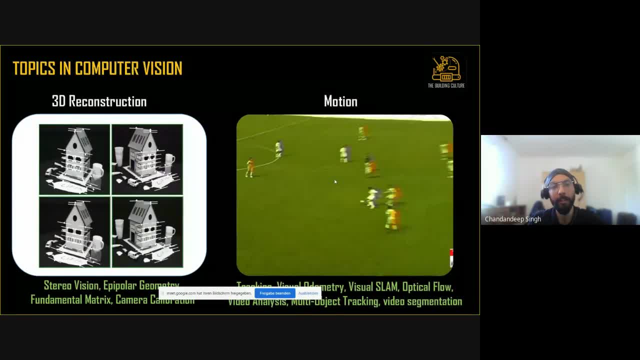 and then what you can do is, once you filter out some of your interests, then you can take up a few projects in that particular domain- and, you know, take up multiple projects- and then you realize, okay, this is cool, but i don't want to, you know, establish a career in this area and then you can explore more. 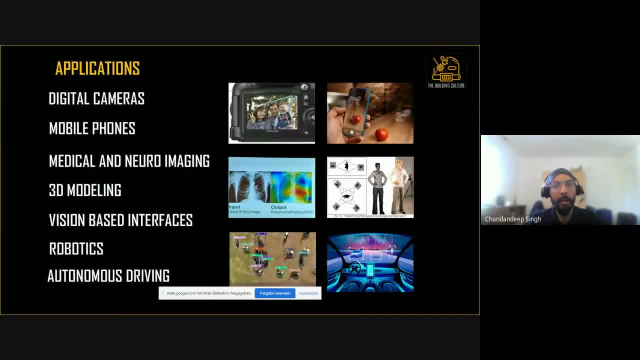 and this is what we will talk about next. but first let's talk about what are the applications of computer vision. so these are just general applications that we all know about. you know computer vision, face detection, face tracking, object detection- all these things are starting to get embedded in digital cameras and also mobile phones- mobile phones, and you know these. 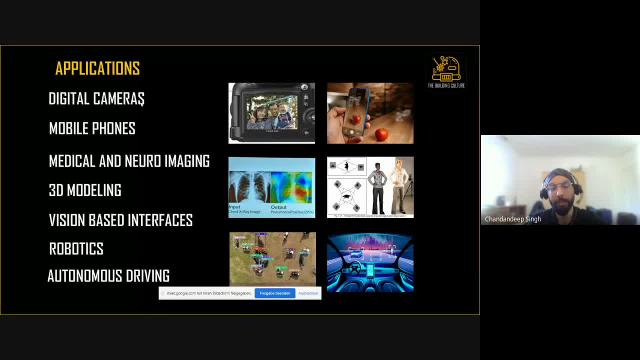 applications on our phones have uh computer vision. a lot of these uh object detection, uh face identification uh applications. use these, this technology, and then we have something uh that is used in uh more in the medical sector uh for identifying uh diseases using x-ray images and so on. it can also be used. 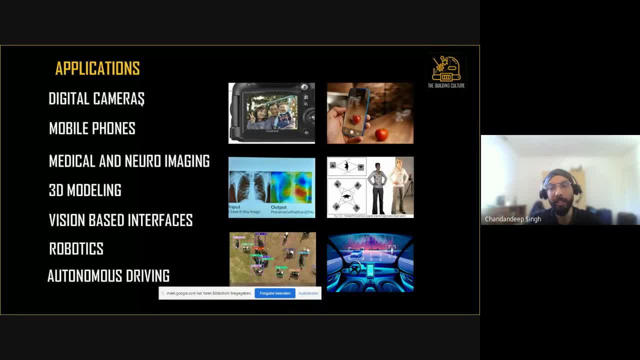 for a 3d modeling, as we talked about 3d reconstruction. it can also be used in movies and so on. uh, then there are vision based interfaces and, of course, it's used in robotics and autonomous uh driving as well. so there are a lot of different applications. these are just giving a broad 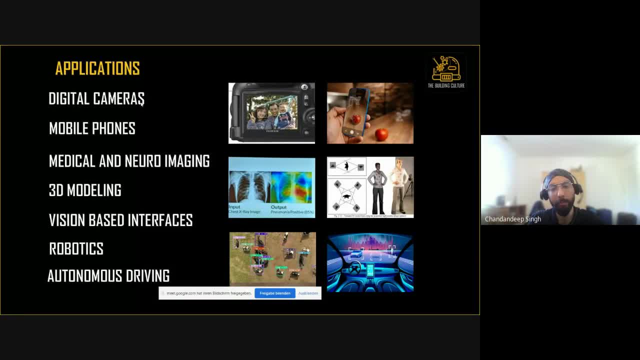 uh, sense of um, these are just to give you a broad idea of what different applications there are, uh, and the reason why this is important to know, uh, the applications, is because, essentially, in the process that i will be sharing, you have to filter out your interest, uh, and for that you have to know what are the. 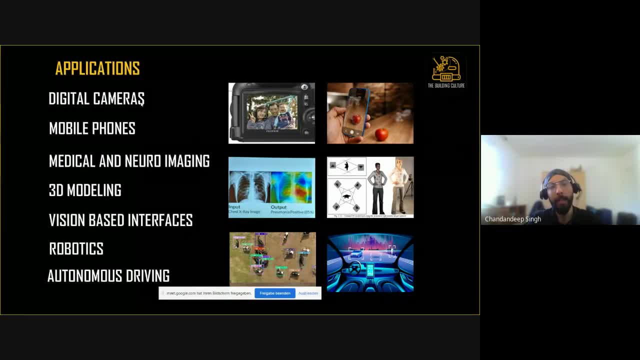 different applications that are existing and so you can choose. okay, yeah, i'm interested in robotics and i want to learn, uh, computer vision for bin picking. or maybe i'm interested in 3d reconstruction and i want to learn more about that. so this is the whole premise of it. now let me talk about how i 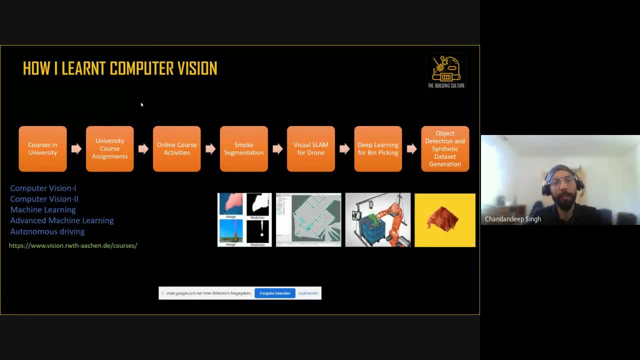 learned computer vision, of course i uh. i was enrolled at a university program at rwth aachen university in robotics and so i got the chance to learn uh in-depth uh theory about computer vision, machine learning and so on, and i took multiple courses uh, but at the same time i took some additional uh. 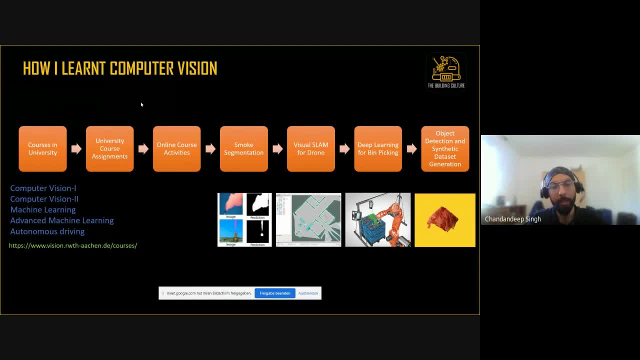 online courses. you know the ones uh by andrew eng, for example, deeplearningai and so on- takes, and probably many of you have already taken as well, uh. so there are two aspects of uh- this university and online course way of learning. one is you, of course, you get a really good. 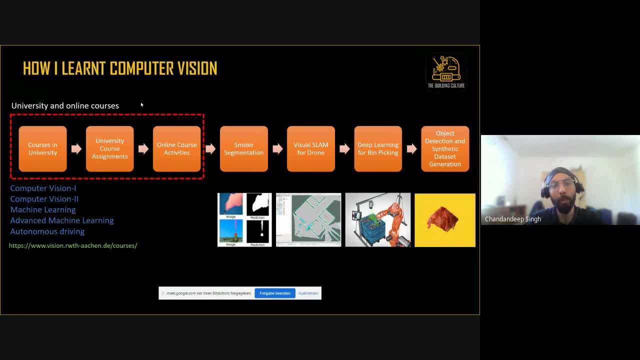 theoretical foundation but at the same time, you have to do lots of activities which are which may or may not be related to real world case studies, but regardless, you have to get your get used to using opencv and all of these uh, uh numpy, all of these packages, basically so i i did a lot of university course. 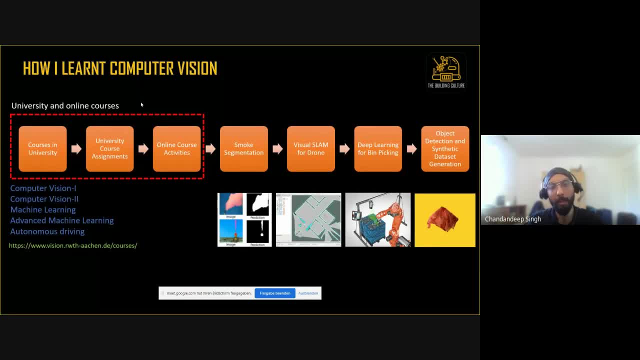 assignments as part of my uh curriculum and i did online courses and also took theoretical courses in my university. but i would say, if if i uh just this part was not uh simply enough for me to you know, uh take computer vision might take computer vision skills to the. 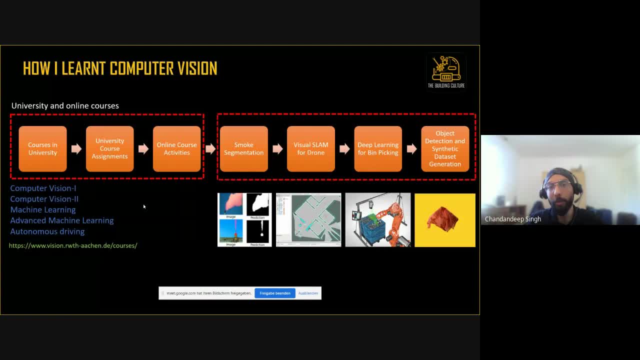 next level or learn even more. so i was fortunate to get some industrial experience, so i worked as a working student in a few companies and then i did internships and my master's thesis, also in similar areas, and this is where i think i learned the most. so one of the very first projects that i did was 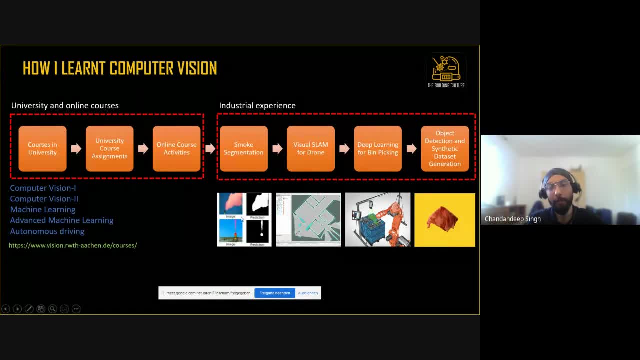 using machine learning, a unit model for smoke segmentation, and another one that i did was to apply a visual slam for a drone using a real sense camera and then after that, during my internship, i did- uh, did- use deep learning and object detection and segmentation models to segment. 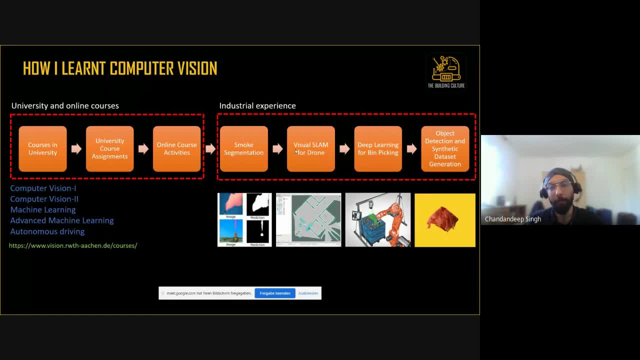 objects inside a heap of objects, basically, and then the robot would pick it based on the grasp points that are generated from these uh objects, uh segments, uh, and then uh. after that i, i did uh some more work in object detection and synthetic data set generation. so this is how i learned uh computer vision basically. and, by the way, 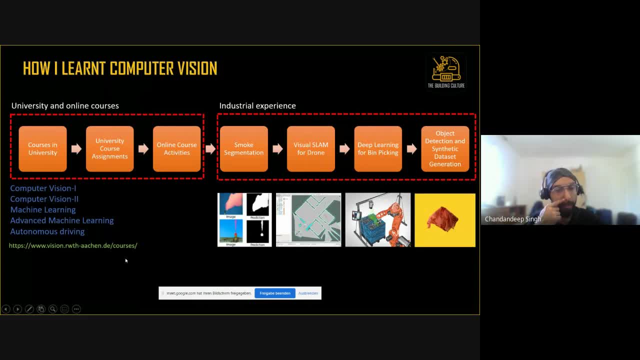 i've also a link to. i've also added a link to the courses at my university. the slides and all are available for free actually, so anyone can start learning and i would say the theoretical slides are really in-depth and they cover the recent research papers. i think they 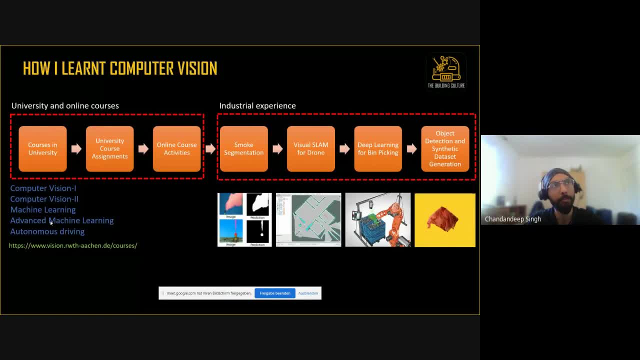 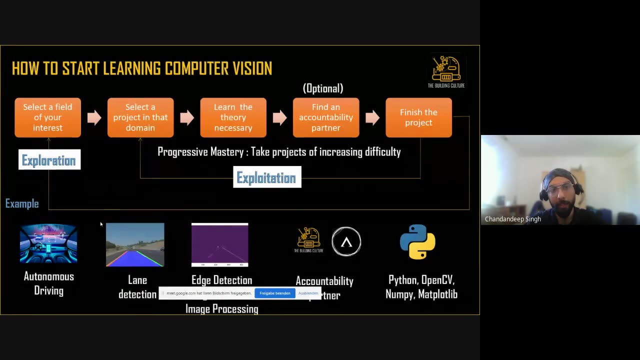 also have slides for all the past years and so on. they they regularly update that as well. so if you are interested, you can also check that. but at the same time i have created a sort of a system or a framework that would help you immediately start learning computer vision after you. 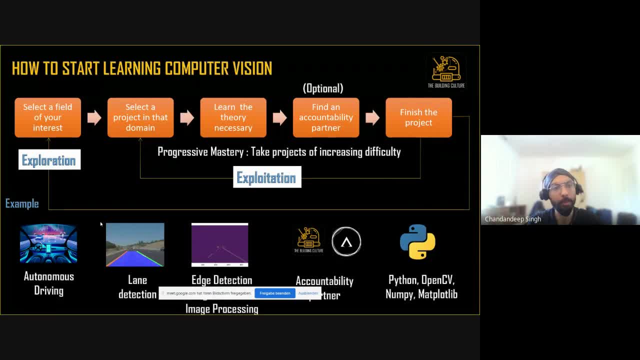 uh, you know, end with this session and go about your day. so, uh, i'm a fan of reinforcement learning and there's this concept called exploration versus exploitation that the reinforcement learning agents go through so as to, you know, have an optimal learning rate to achieve the desired outcome. so this is what i try to apply in my own way of learning as well. so 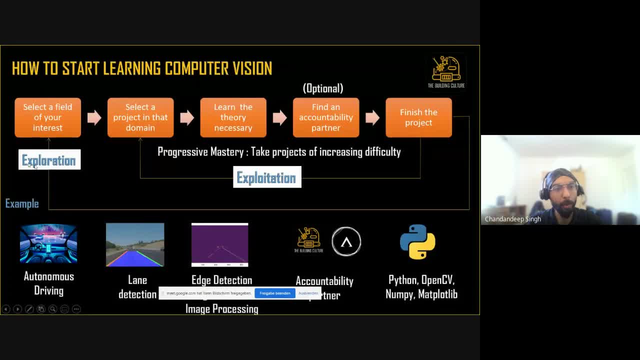 the framework that i'm using is that of exploring, uh your interests first, and once you uh once you have explored enough and you realize that, okay, uh, autonomous driving, let's say, is the area that i'm interested in, and then you take up more and more projects, uh, in a progressively uh increasing. 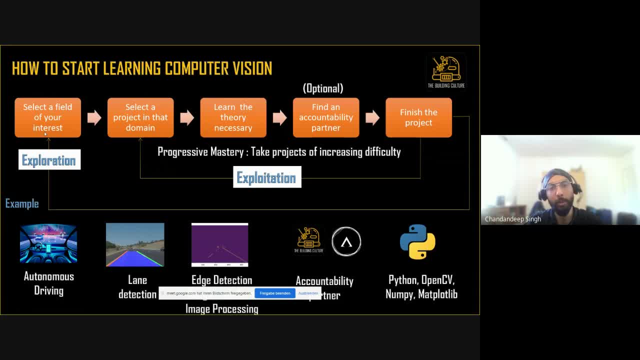 uh, difficulty, uh way, such that you, you, you can gain mastery in one area. and here i would also like to point that, uh, eventually you know to get a job, or you know even to do a phd or whatever, you have to have one area where you are really good at and, of course, having some 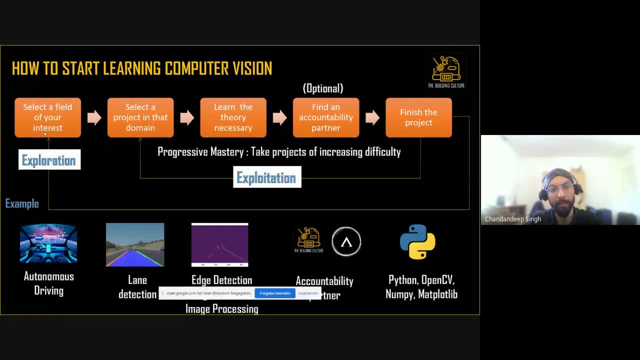 overall view of all the different uh areas is also essential, but you have to have a specialization, is is what i mean. so let's say you are a total beginner and you want to learn computer vision. how start? so the first is uh selecting a field of your interest. how would you select a field of your? 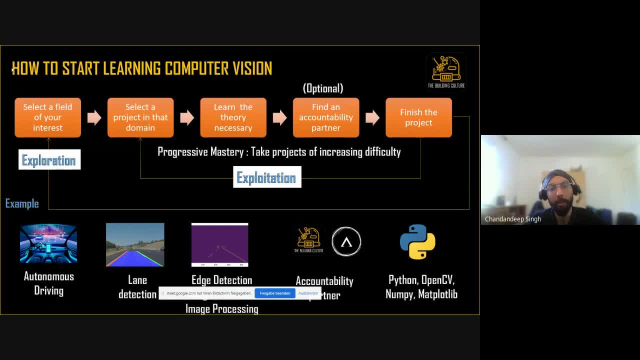 interest at first, you, you, you probably don't know which area you are interested in, right, but you see these videos on youtube and you attend these seminars and you talk to people and so you realize that, okay, let's say, robotics is something, uh, computer vision for drones is something i would be interested in, for example. so what you do is you just 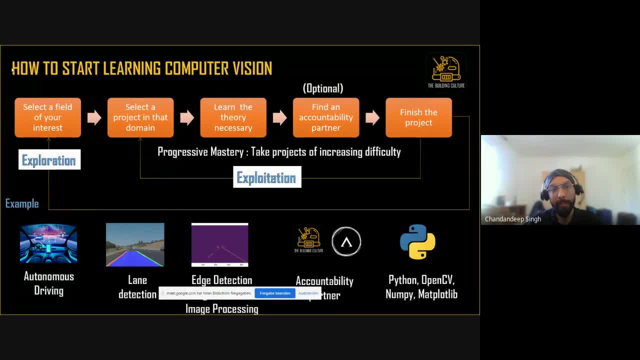 choose a project in that domain and then then you learn the necessary theory, and for that you there's plenty of uh information online, and once you have learned the necessary theory, you can start working on the project. another optional thing that you can do is you can find: 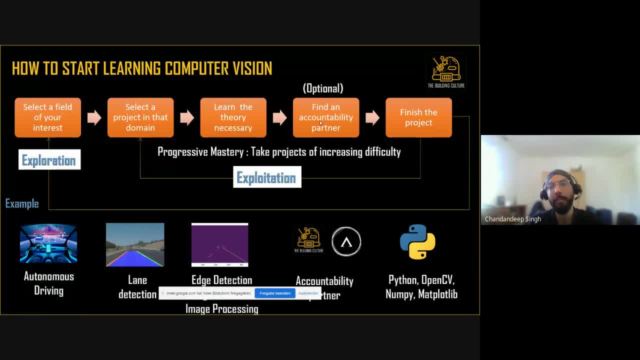 an accountability partner. you can talk to your friends or go on to these discord servers or facebook groups or whatever. you can find people who are also starting out and you can, you know, help each other out when you're stuck. and once you finish the project, then is where you have to take, you have to pause and 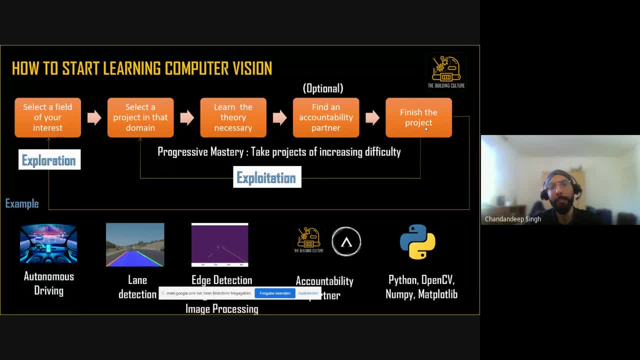 you have to think, uh, is this an area where i am interested in, where i would like to learn more about? are you excited by that uh project or the domain that you chose? and if you did, then what you do is you would take up up another project. so another thing to point is that you select a very simple project in the 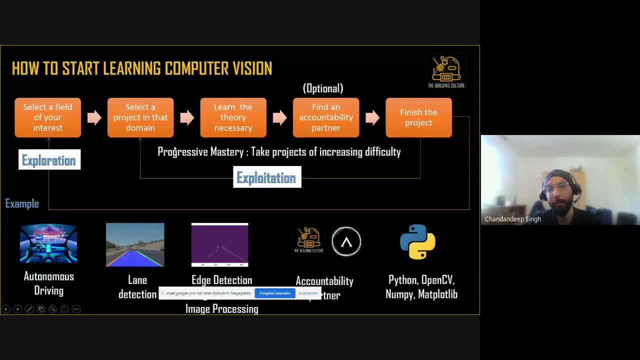 beginning, and once you like it, then you, then you take up another project of a slightly more difficulty and then, if you like it again, then you, you know, you, you could eventually, you know, be increasing your skill level, uh after uh, every project that you do and maybe, maybe you don't. 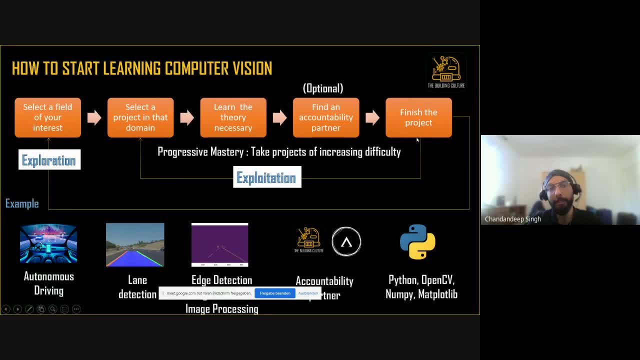 like the uh the thing that you did. maybe you realize that there's not a lot of uh opportunities there, or maybe you're just not interested in uh the project that you did. so you, you go back to the first step and you explore more. you, maybe now you take a different project, maybe in uh medical image. 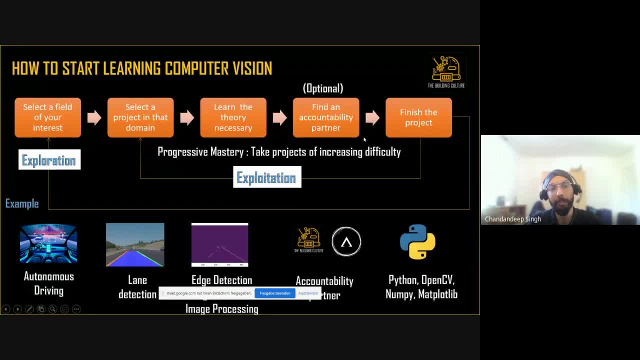 processing or something, and and you repeat it: the same, uh, the same way. so let's take an example. so autonomous driving is something that uh is, you know, growing very rapidly and we see it uh everywhere with with Tesla and uh other autonomous uh driving companies. you know making these announcements about progresses in this area. 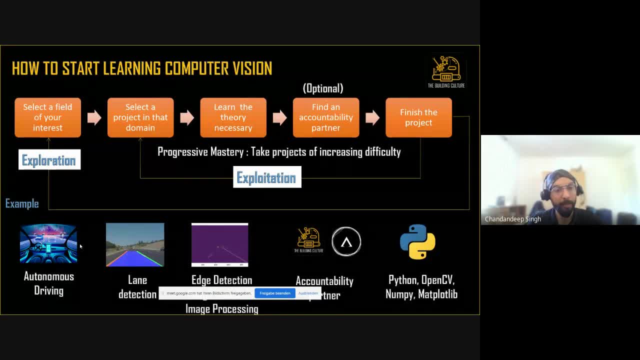 so you say, okay, I'm interested in autonomous driving, uh, and then you take up a very simplistic project, uh project and, of course, for that, how do you know the projects that uh you have to select? uh, to keep to take a very simple project- and I'll talk about, uh, how to select projects in the next. 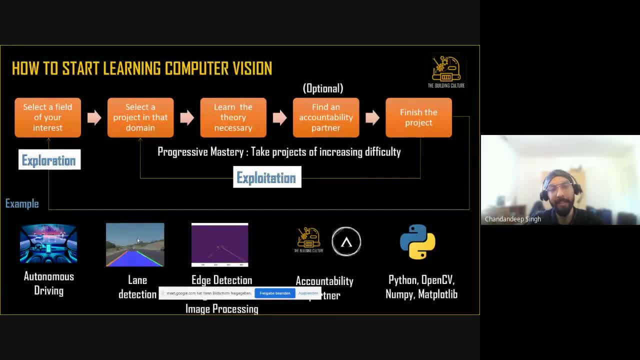 slide as well. but the idea is to keep the project as simple as possible, uh, in the beginning, and not to make it too complex, because if you take up a project that your skill level is not sufficient in, you would lose motivation, because even in simpler projects you might get stuck in the beginning. 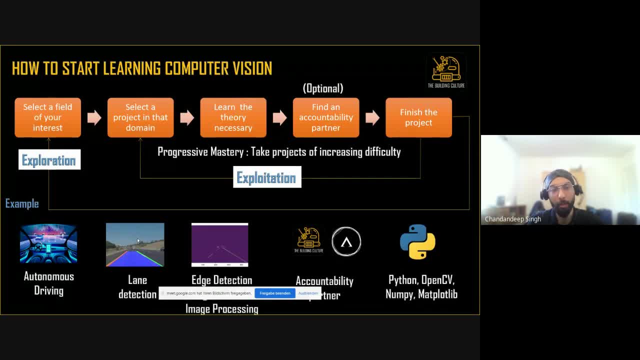 uh, and let's say you, you take a plane detection now you, you search online and you realize that you need to learn some theoretical concepts, like it would maybe require basic image processing, like edge detection, hog transform and these things. so you just learn the bare minimum concepts that you need to learn and after that maybe you select an. 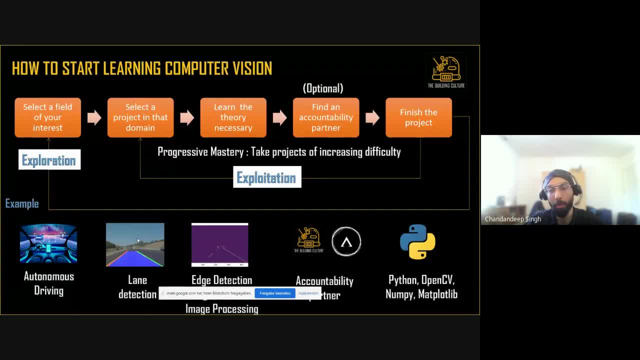 accountability partner, or this is an optional step. you can go on to servers like alpha bot robotics or the building culture community or Facebook groups, or you can talk to friends and so on. you can choose an accountability partner as well if you want, and then you start doing the project. now, I mean it's it's really simple to find, uh. 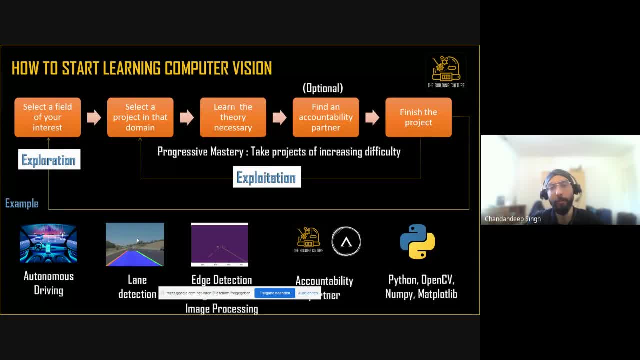 tutorials on these simple projects, you. you can find open CV tutorials. there are other resources that are also shared online, uh, but the idea is: you don't get to, you, don't you know? uh, hang up too much on the theory, you. you start to apply these things immediately. for example, 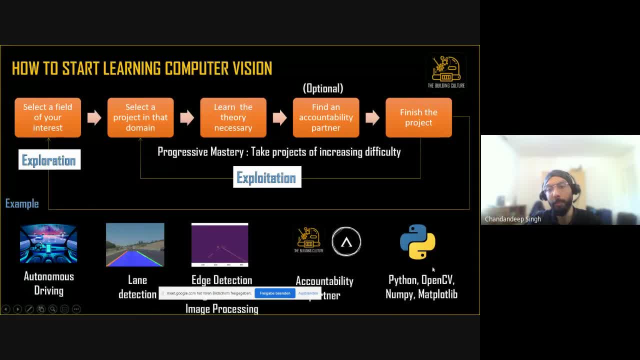 there would be packages- uh for edge detection in open CV and uh you. the idea is to start coding immediately and then if you see, okay, there's a some there, I need some more Theory, then you go back and you know, uh, watch a few videos as well. so this is my approach overall, how you can start. 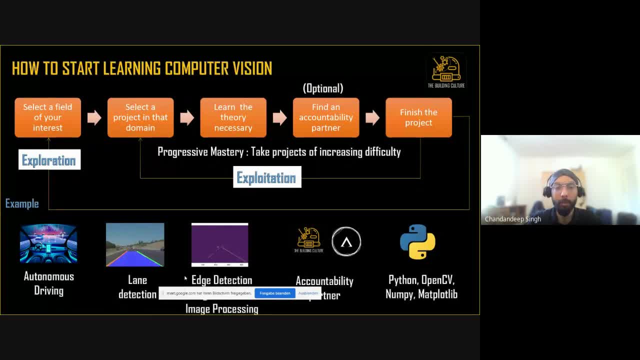 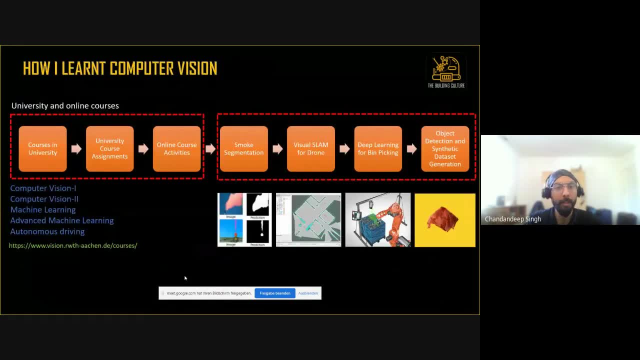 learning, computer vision. now there are a lot of people who would say that you should take the first step and have a really strong theoretical Foundation in, uh, all of these areas. of course you can do that if you have the time. uh, but, uh. but this framework that I'm providing is uh, more. 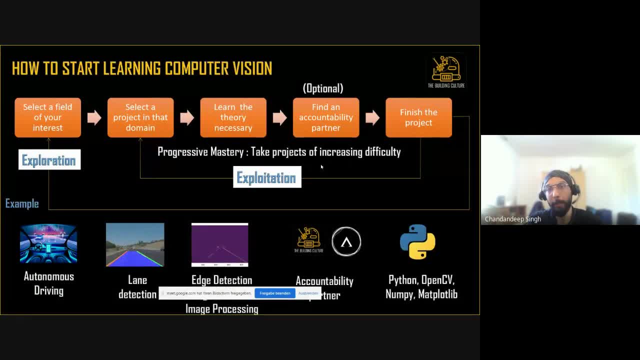 efficient because you can start to do hands-on work- uh, more immediately, of course. and also, I'm also curious what you uh, what difficulties you face while learning, and um and uh uh. what do you think about this framework, if it will be useful or not. so let's not talk about how to. 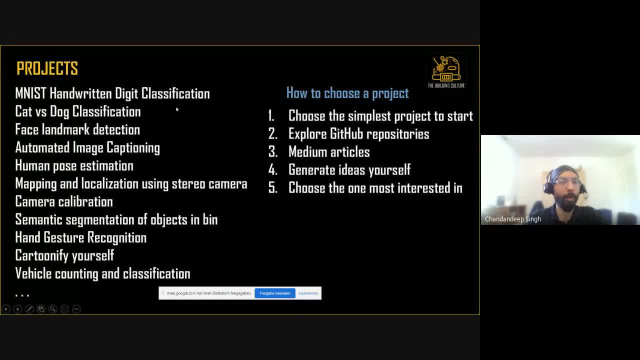 select projects. so these are just a bunch of projects that are very commonly used, of course: cat, dog classification and MNIST. handwritten digit record- uh digit classification, and face landmark- uh facial landmark detection, automated image captioning, pose estimation, camera calibration, segmentation of objects in bin, cartoonifying yourself, and so on. I mean, the list is endless. 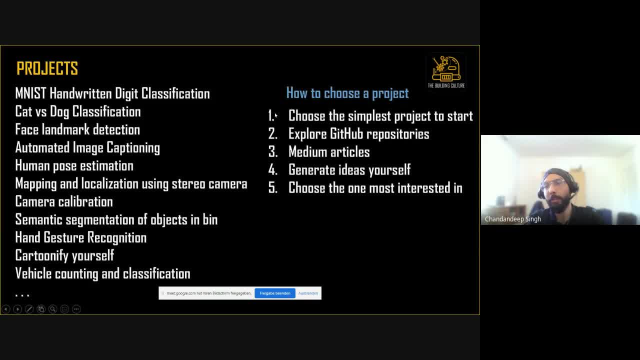 but the idea again is to choose the simplest project to start. you can explore GitHub repositories, you can check medium articles, you can just simply Google it right there you will find a bunch of information. but you choose a project and then you stick with it. uh, another thing that I like to do is 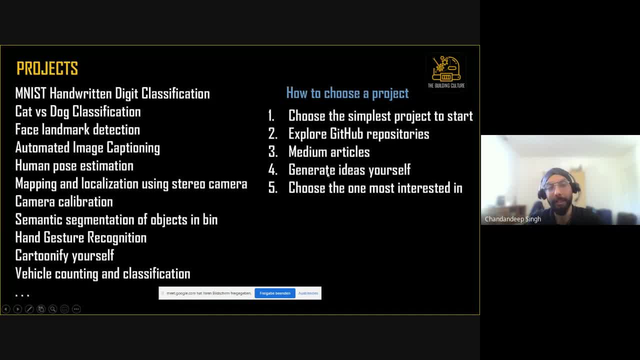 uh to generate ideas myself, so you can generate, uh, your own ideas, project ideas. so, for example, you work on your laptop and you think, okay, uh, what if there's an app called app that actually helps you? uh, pause uh your music player without using the keyboard so you can use your laptop camera to, let's say, do a gesture recognition, or 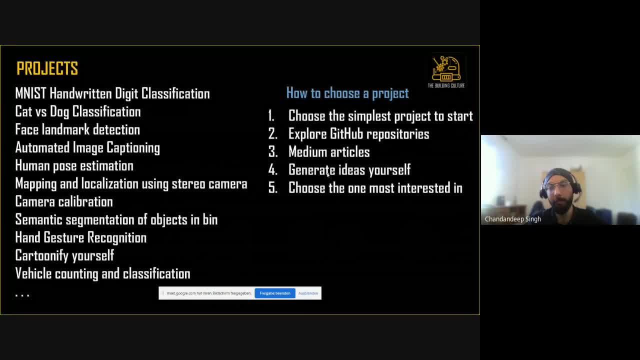 something uh to build such a system. now there's already an app like that called Flutter. you might know about that, but you can come up with your own ideas, and the reason why I encourage you to come up with your own ideas is because you would be uh excited to do the project and you're 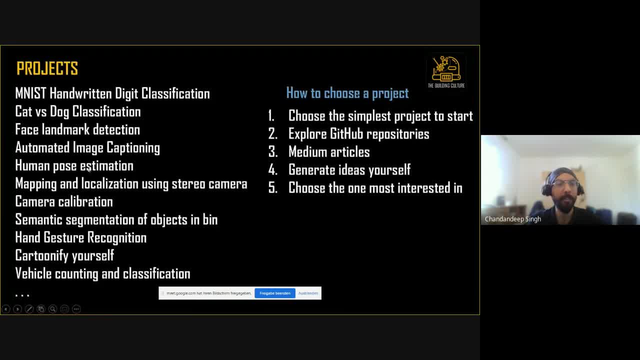 more likely to finish it otherwise randomly. if you select, let's say, human pose estimation, and you get stuck or your accuracy is not enough, then you might lose motivation. so this is another thing that you can consider. of course, you can also Google search your projects, primary ideas, choosing a very simple project in the beginning and choosing the project you're. 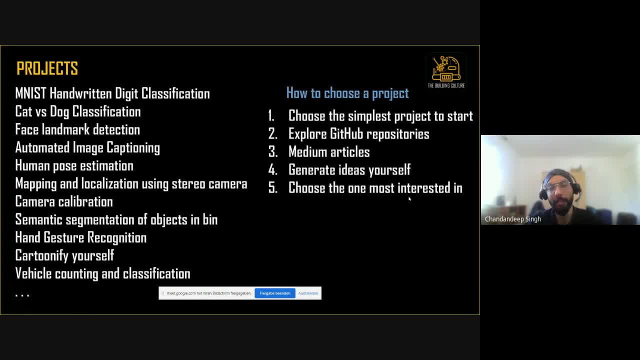 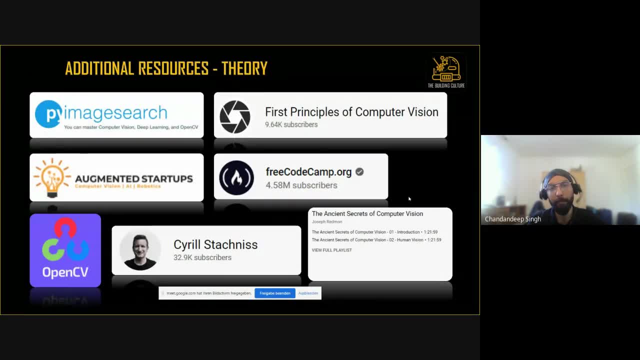 more most interested in. so choose a project you're interested in. that is simple enough as well. now there's a lot of so it's not just for theory. i've written additional resources, theory it's actually some of these resources. you can start to use uh for your projects immediately. so, talking about theory, so there's uh, these couple of youtube. 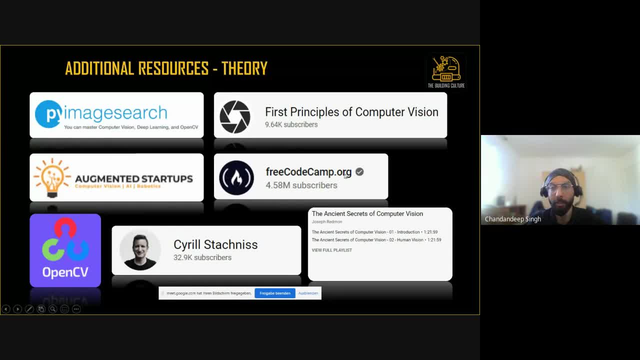 channels that you know about free code camp. it's actually also a very hands-on, tutorial based way of learning. they have some tutorials on computer vision and then first principles of computer vision. this is a more of a theoretical, lecture based learning, and then there's these: uh proper. 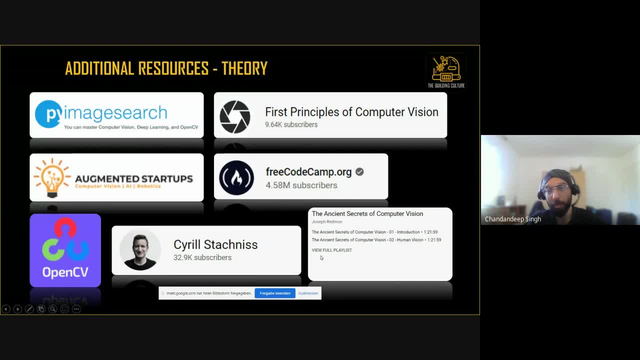 lectures called at uh ancient secrets of computer vision that you can check. uh, of course there's this, uh, professor cyril starkness from university of bonn. you can find his lectures as well online. i used to refer them. they're very detailed, so, especially if you want to. 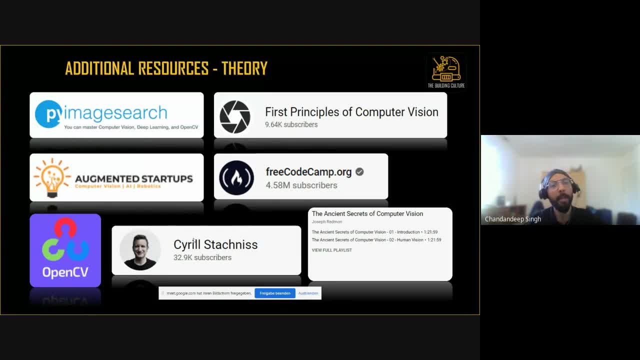 go into research, these lectures would be helpful, but if you want to just get started doing uh, get started with doing projects, i think. for me personally, i found this uh pyramid search as the best resource where you can start to use opencv, computer vision and deep learning, because they have very structured, step-by-step 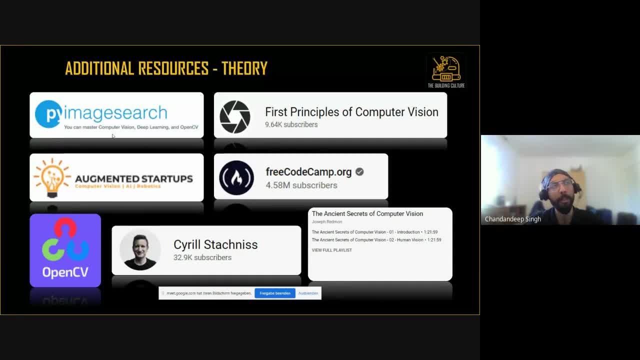 guidelines on how to start doing a project even. they even have tutorials on installation of opencv and and its dependencies, because initially that could also be a problem. and another one is augmented startups- uh, this is another good website. they have a youtube channel as well and they teach how to build projects, how to use different models, yolo mask, rcn, and so on. so 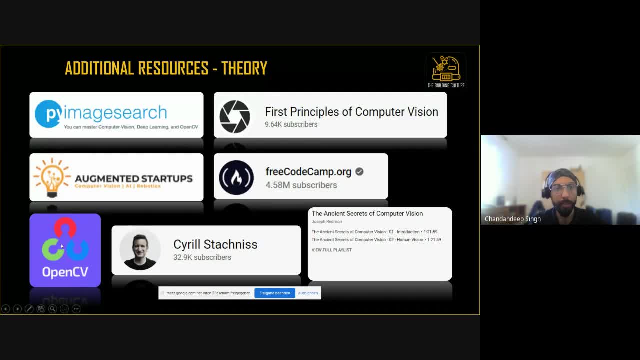 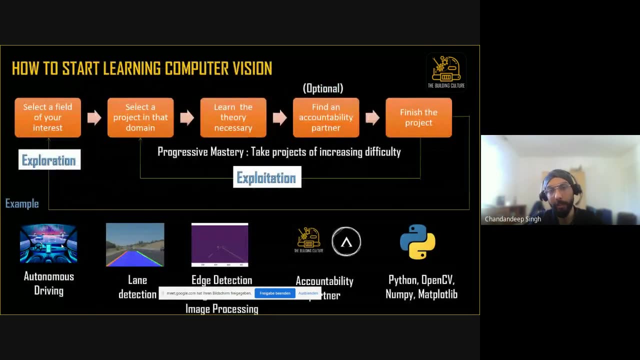 and, of course, you can go directly with opencv tutorials. it's very detailed and very hands-on, so these are some additional resources that you can uh refer to. but again, uh, my view would be to take a project of your choice and progressively increase in its uh increase your. 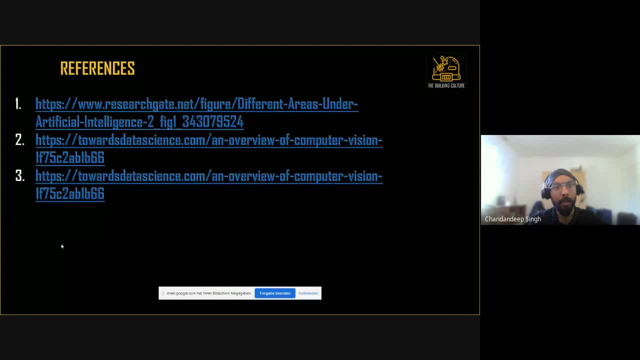 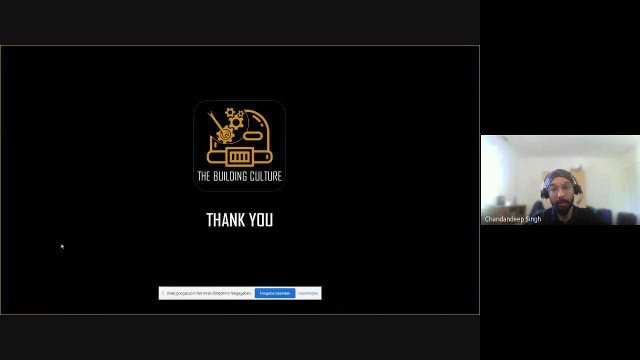 skill level and and the difficulty of the project. uh, and these are some of the references that i used in making this presentation. uh, i think there were more references but i couldn't add it. but i i'll add it later and maybe share it back with you. so that's it, uh, from my side, and, if you have any, 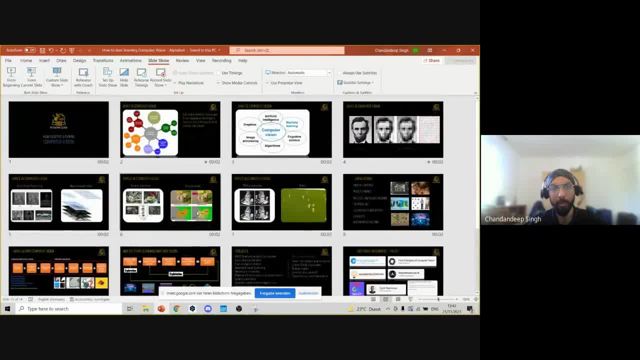 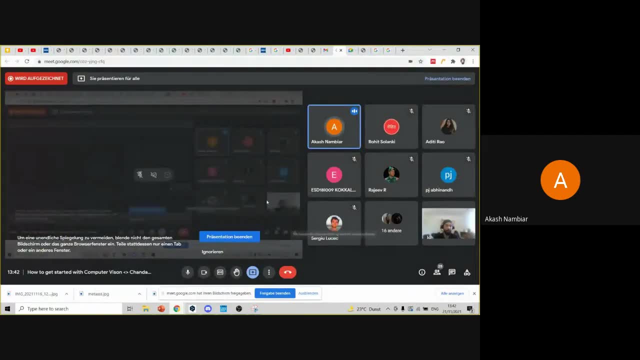 questions related to any of the slides or anything. we can talk about it wonderful, like, uh, anyone, uh, anyone has any questions regarding computer vision, or if someone is yet to get started with computer vision or someone is already into computer vision. you still have, uh, you know, some roadblocks that you would like to discuss with sendeep. 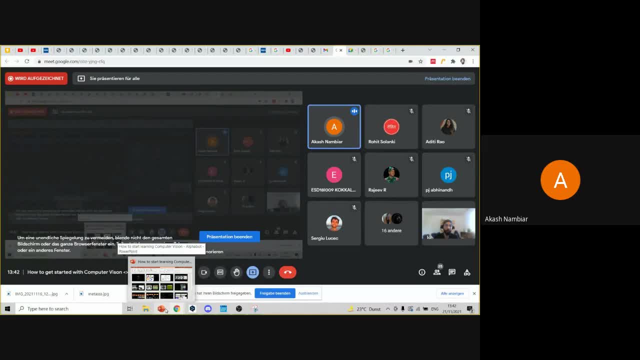 in fact, we can all come together and maybe we can have a good discussion right now. it would be a good chance we could discuss a lot of cool things right now. anyone, uh, anyone with hello, sir, yes, yes, go ahead, uh. so my question is, sir uh, so if i start the, the computer vision, with the 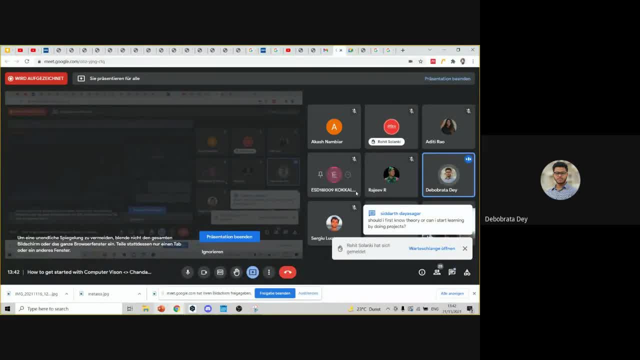 robotics. so, uh, just assume, sir, i build it the the. that's one robotic arm and i want to implement the computer reason with it. so maybe i uh obtain by this robotic so how i control the robotic. uh, so your question is that you have a robotic arm but you want to 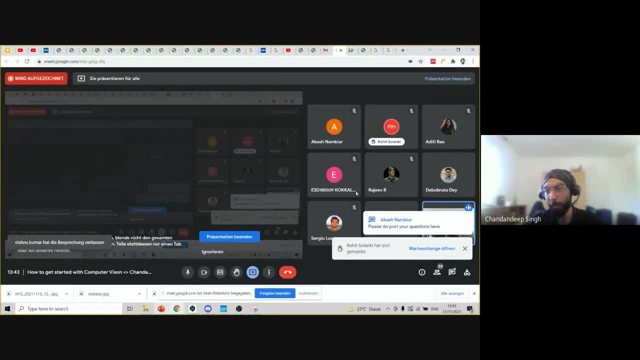 control the joint movements, uh, using computer vision, right, yes, yes, yeah, so you can use some uh specific approaches like visual surveying. uh, you can google it or so. the idea is that it has to be an integration of computer vision and control. so visual surveying is one, a really good option that you can consider. but do you have you? 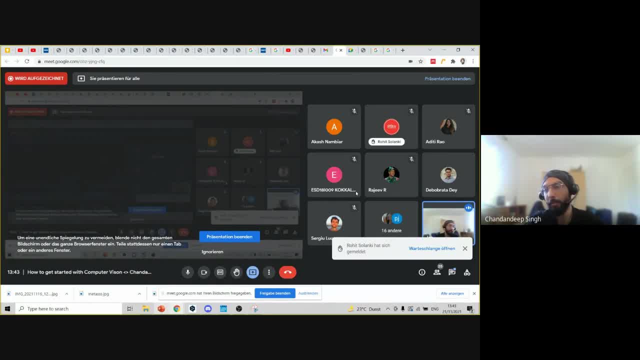 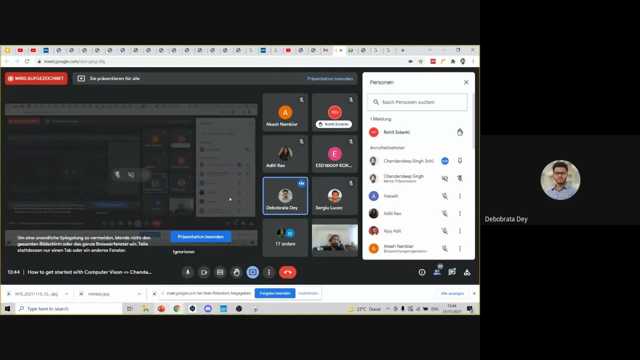 built the hardware yourself, or you're using a kit, or what exactly are you using? uh, sir, i just you know the uh, the starting state. sir, i build the hardware, but, sir, i stuck in the this, uh, implement the computer vision part. okay, okay, okay, and have you done some computer vision? 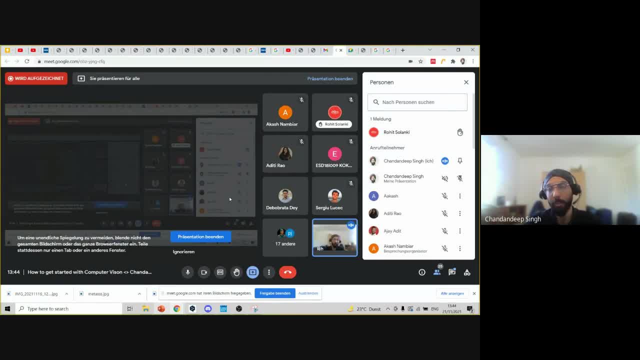 uh projects before, or is it? uh just, you want to start with it using this? yes, uh, sir, by keyscat file. so so, just, i am the bb beginner on this domain, sir, so i just uh use the hard cascade file, so uh, to uh detect some object in various object, like, uh, if they are one card. so i just put. 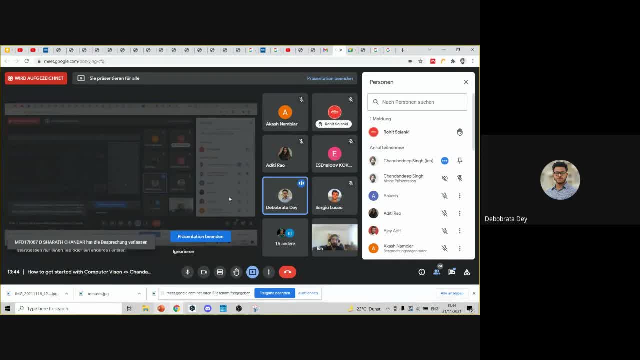 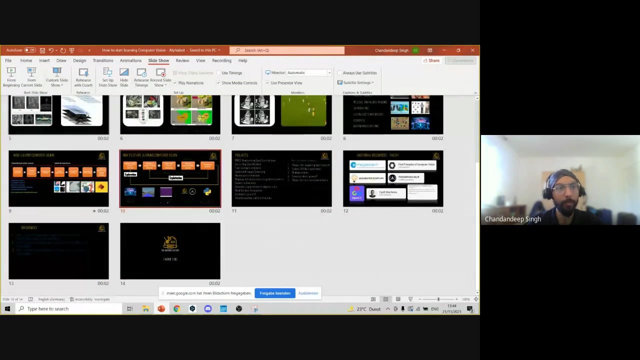 some picture with the hard cascade file and they detect the just one card is there like that only okay, okay, okay, okay, yeah, uh, so, but you, you, you want to work, you want to explore the robotics, uh, computer vision for robotics area. basically right, so, uh, yeah, so, basically uh. let me share the screen where i was talking about the framework. 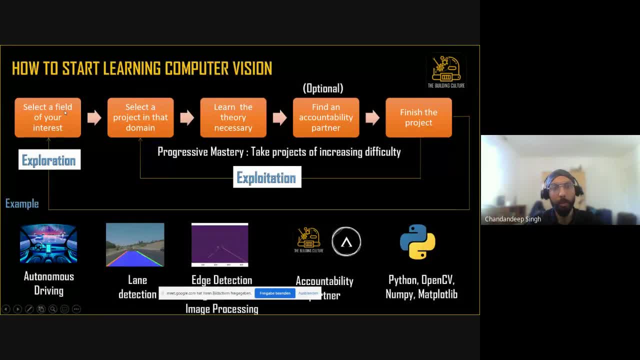 yeah, so. so here your interest is in robotics, right, and you want to uh use uh computer vision, uh to actually control the robotic arm. so what exactly do you want to do? so the camera would be mounted? first of all, you have to figure out the hardware arrangement, i think. 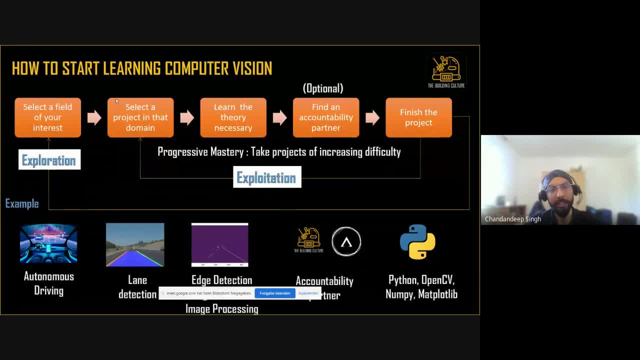 so that you can define the problem. uh, so is the camera on the end effector? uh, and then you want to? sorry, so i just mount the camera on the end effector. okay, okay, okay, and uh, what exactly do you want to do? so you want to, uh. 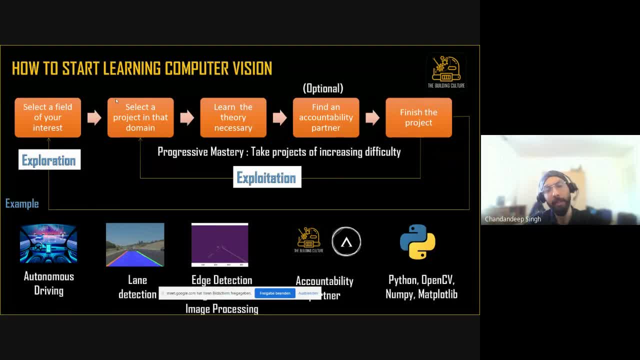 capture images- uh, from the end effector, uh camera, and then, uh, what exactly do you want the robot? do you want the robot arm to track an object and move accordingly, or what specifically do you want to do so? first of all, my project is the- uh, it is the harvesting robotic answer. 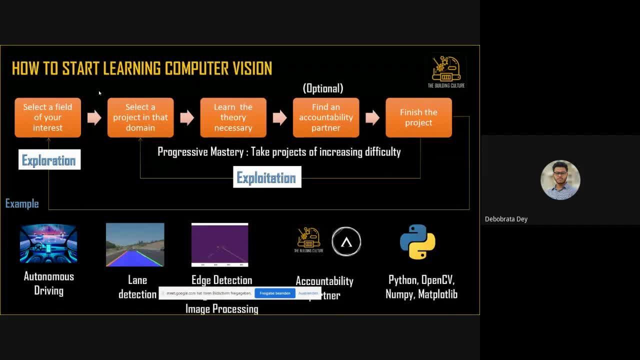 okay, okay, yeah, so, uh, so, if there is a one flower in one tree, sir, so my aim is to find out the coordinate of this flower by this robotic arm and the camera also. okay, and uh, yeah, and then the robotic joint movement also to plug the flower from the tree. 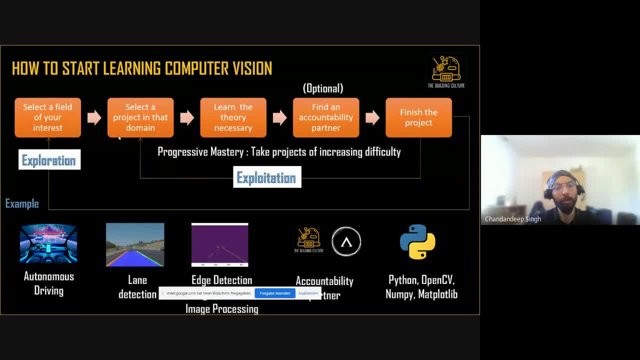 like this: okay, okay, okay. so the? so what you are telling is actually not using computer vision to uh, control the robotic armamp. I think that's a different visual serving is not what you need here. So what you would be doing is basically using deep learning for object detection. 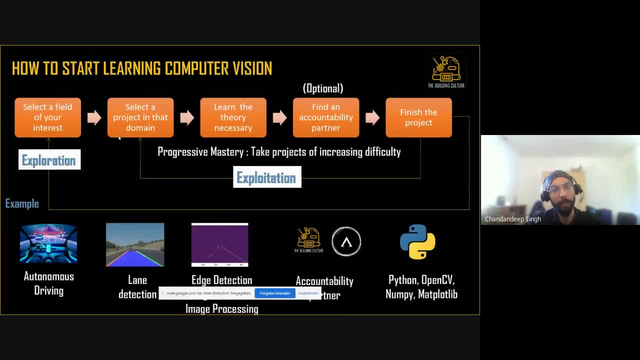 So let's say we have a flower, right? So you'd be using deep learning for detection of that object and then eventually find. But yeah, so here you have to figure out the hardware first, because you also want to have a gripper, right? 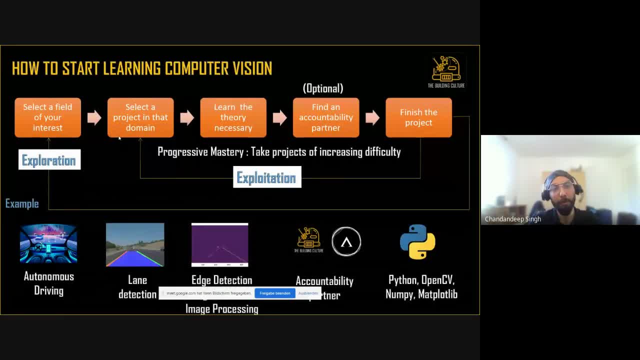 So how are you going to arrange that? So I think the first step for you would be to define your project very clearly: whether you really want the camera on the end effector or can you place it externally, Because for harvesting type of projects, 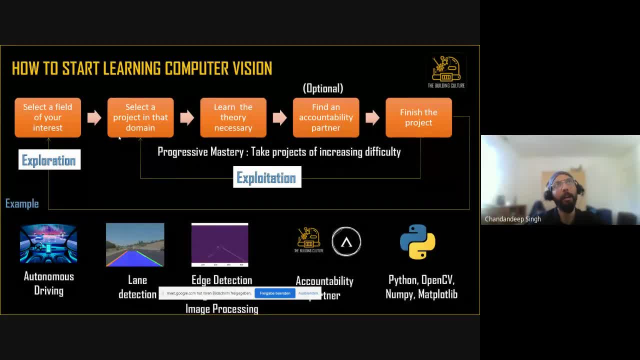 what is generally done is they make the camera, let's say, overhead. It's mounted in a fixed way. So just imagine the camera is mounted overhead and let's say we have a plant or something and we have flowers on that, And then the robot end effector has the gripper. actually, 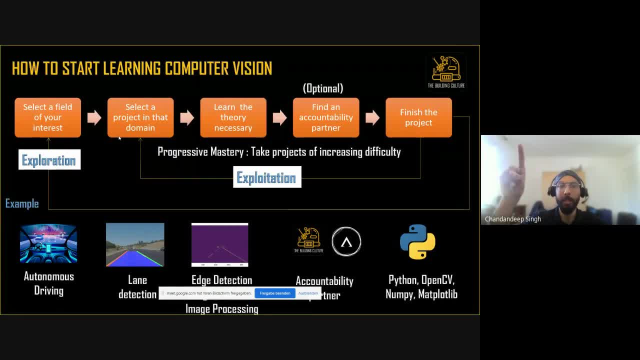 Not the camera. Right So you would use the camera, The images captured from the camera, to train a network to identify flowers. Right So you would use supervised learning for that and you would label those images and feed it to the network and then 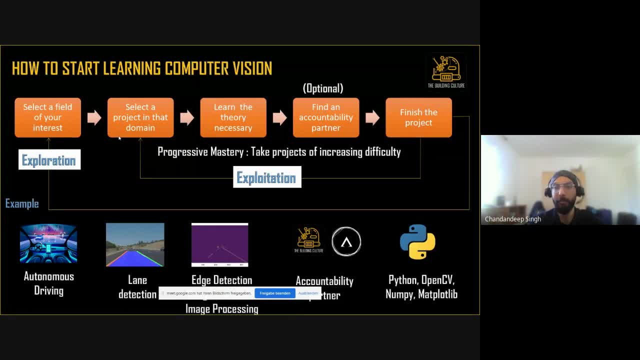 then after that, what you would do is, once you have, let's say, a flower, then you would pick out, Then you would find the grasping point using the, the, the detected object or the segmented flower. Right, Once you have the grasp point, 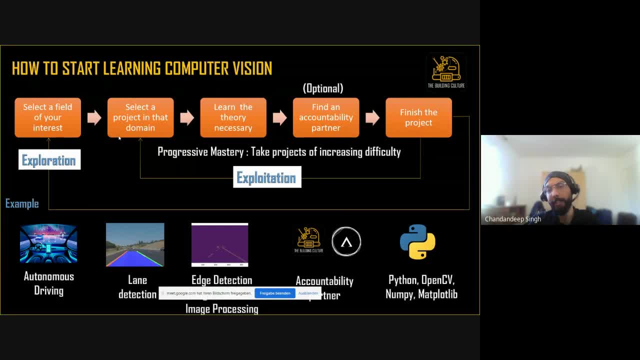 then you would feed it to the robot and then then would be the control bar. So here the control and computer vision are not working simultaneously in this case. Does it make sense? Yes, sir, I got it So, but this is the project that you want to do, right? 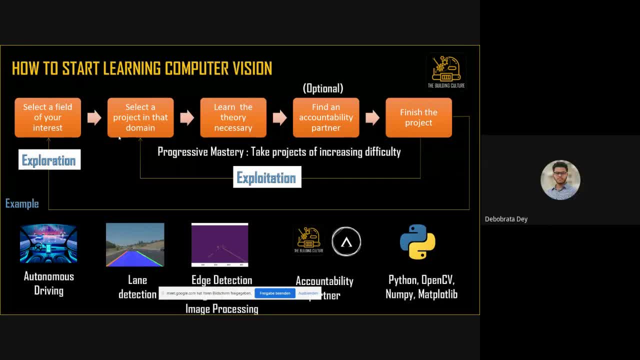 Or Also, I already- mean I already built the project actually, but I did not completed the computer vision parts. So OK, OK, But this is exactly what you want to do, right With harvesting, it identifies and then grasp, point and picking right. 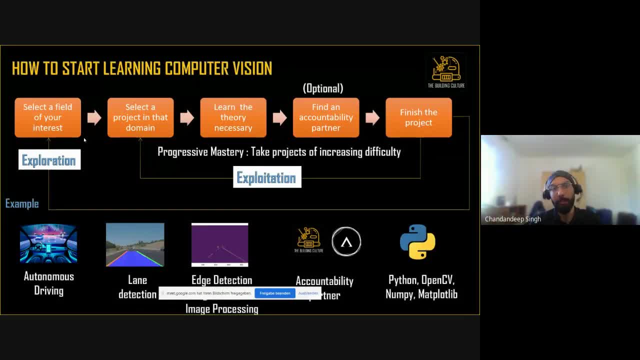 Yes, sir, Yeah. So yeah, the first step would be to decide actually where you want to place the camera, like setting the hardware stuff, fixing it fully, And then you go on to the computer vision part And you forget about grasping altogether. 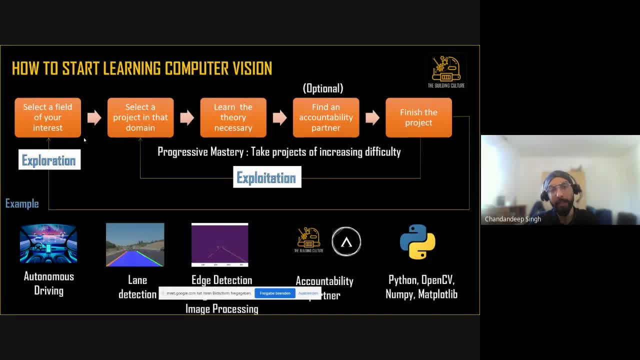 Right. Of course you have to take that into account as well, But you first focus on training a model to identify the flowers and then how you can use the output of the model, let's say if it's a segmentation or object detection or 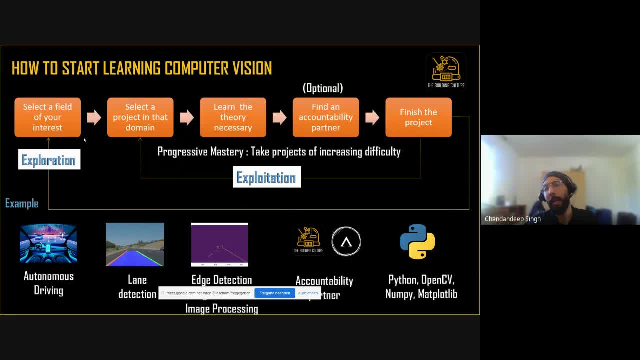 a contour. whatever you're getting you get. you try to get a grasp point from that And then you do the grasping by the robot. So just break it down into three or four parts, Otherwise it gets confusing, Right? So yeah, just yeah. 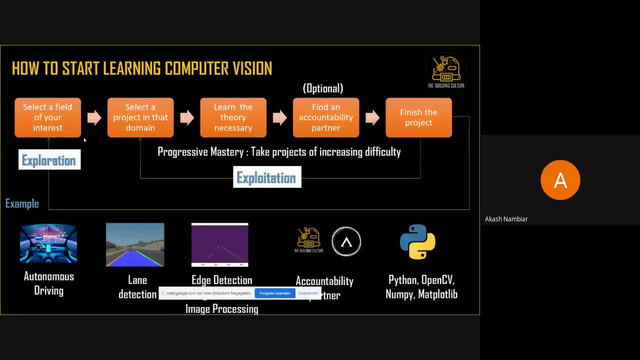 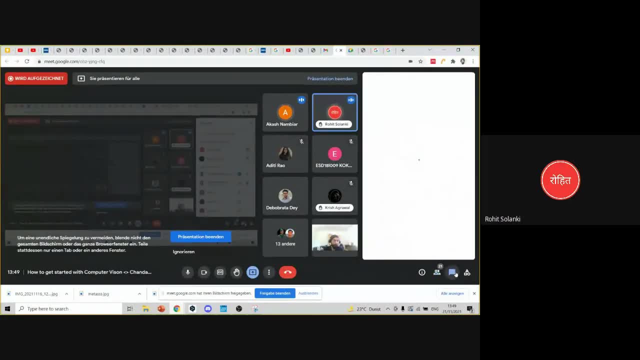 And then I think we go ahead with other questions. I think there's a few questions, So yeah, with that, what is this idea? Yeah, Please, let me know if I'm audible. Yeah, yeah, Yeah, I'm trying to train. 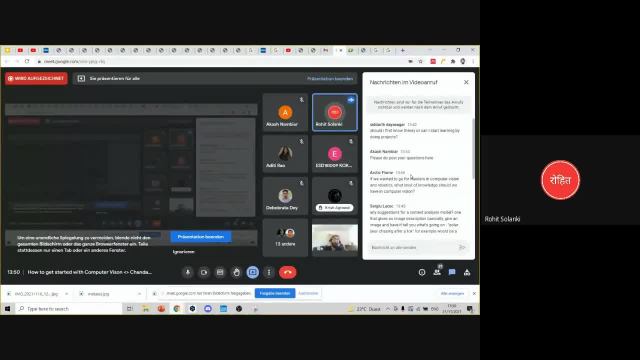 So hello sir. Actually I started a project In computer vision around six or seven months back And at that time I got a real hard failure in that because the project was to, it was related to semantic segmentation and I was expected to use mask RCN in that. 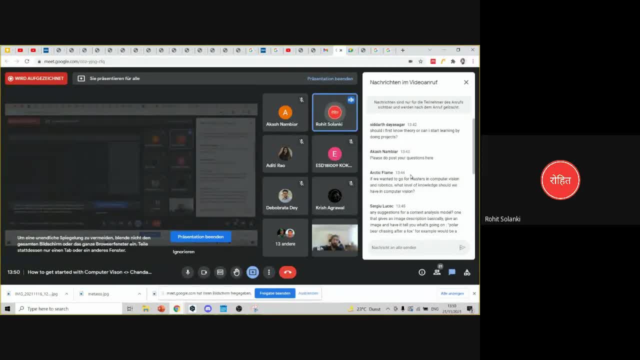 But my knowledge on deep learning and computer vision wasn't enough. So I was very much heartfelt kind of person so I took on- I mean I gave up on that project and I went on with embedded systems. I did some internships and all. 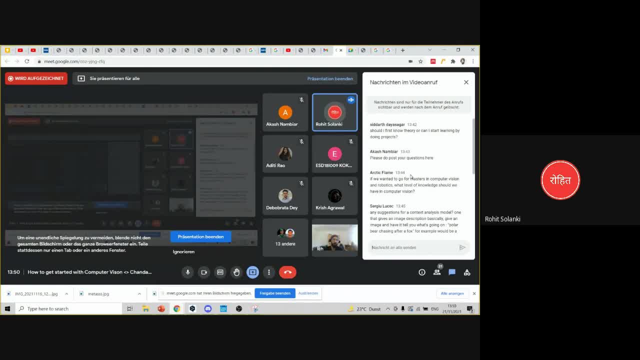 And then I decided to take a break because I was completely confused what to do. I mean a lot of knowledge of a lot of fields, But I was complete My I don't. They won in each foundation, if you know about that. 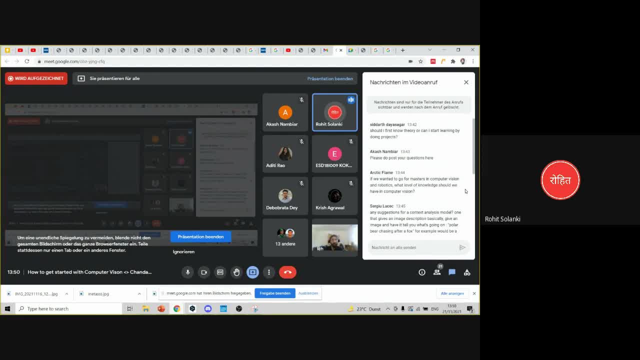 And I just came out of the foundation and I was thinking of going with the mobile robots- means my main interest, I think, is not. I think I just means went through all the means. I just see in my past that what I have done and what are the what are, what are. 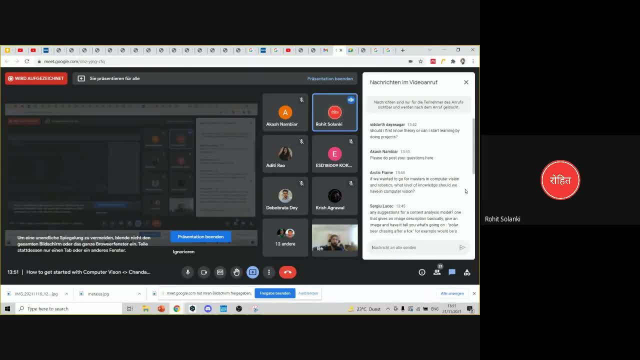 the all the mistakes means, as you told us, that don't take a big project. You will be get, you will get confused and you will be very much heartfelt kind of thing. So those things happen with me and with projects also. I was choosing big projects, not focusing on basics. 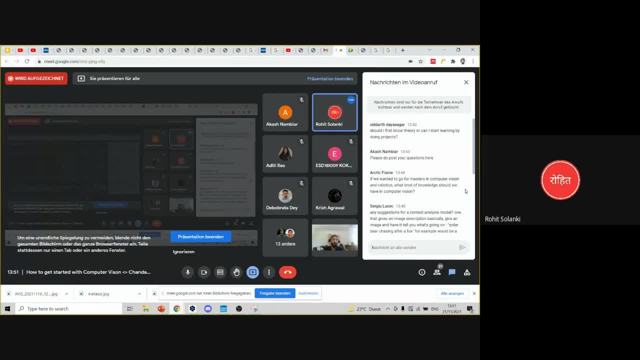 So that I am planning to do But I realized is that I want to go with means, mobile robots and slam motion motion planning and computer vision in motion planning especially. I want to go with that. So I have three things in my hand. 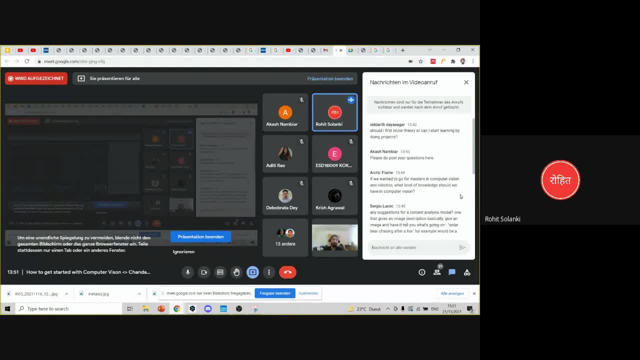 Actually, I have a project which was provided to me from the community- It was this same project which I was talking about- that I have to use my mask and CNN to calculate the number of vehicles. So that thing I want to do, that I have. 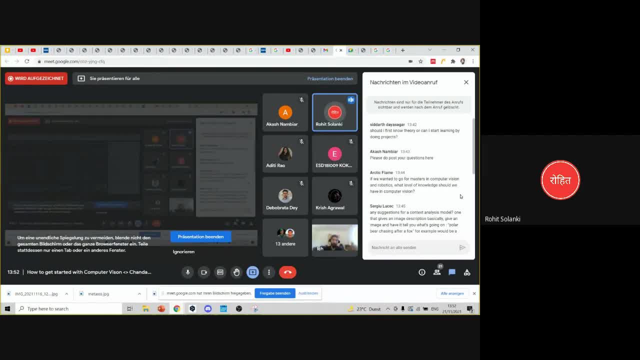 So I Participated in a kind of competition. It was from NXP and it was named as artificial intelligence and mobility. So I have a simulated problem statement in which we are given a card and we have to like use for this computer vision to break the path and object detects and 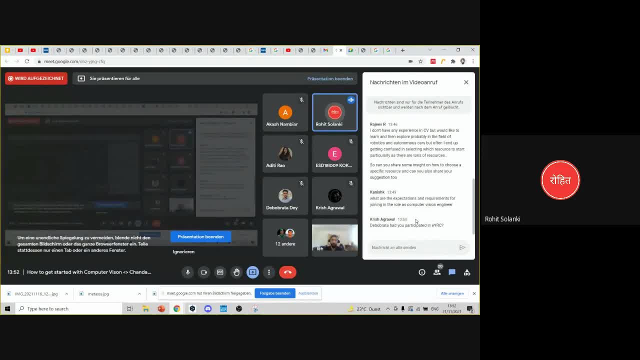 to complete the trajectory in a given amount of time and In a manner. So I want to do all these projects after I go home and start doing my project. So I think my this is the means. this is the first meeting after I am coming out of the break. 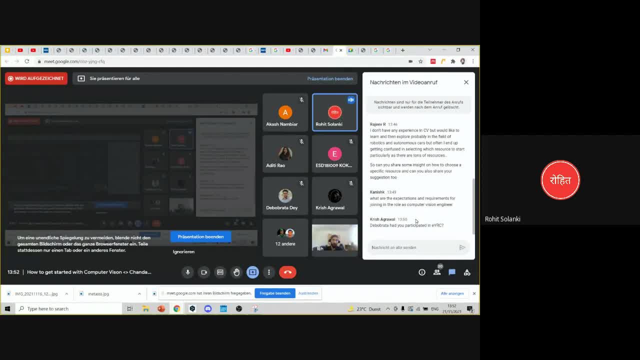 So it was my great pleasure to have a mentor like you at the first, So could you please guide me with that, OK, thanks. Thanks for sharing your overall journey. Basically, What I understand is actually: there's a lot of noise. Oh, I'm sorry. 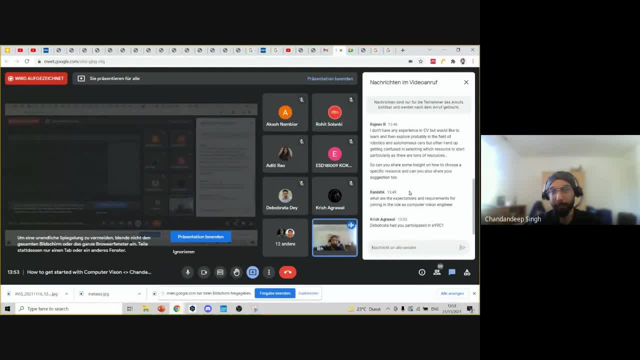 Yeah, what I understood is that you want to learn mobile robots and you have a lot of project ideas that you want to learn, but you take up bigger projects and then you get stuck on that, Right? So, yeah, I mean, my suggestion would be to take 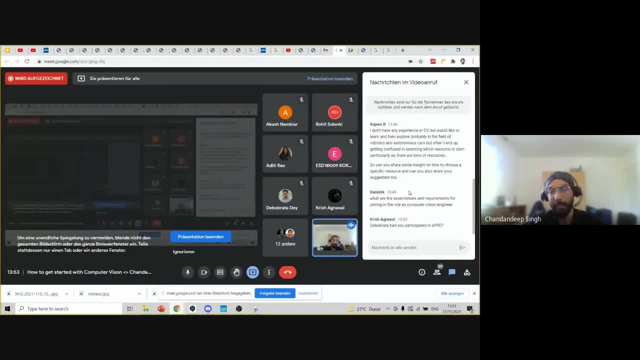 a simpler project, or if you want to take a big project, to have at least a few friends with whom you can do that, so that when you get stuck, at least you can get a different perspective. and another thing about mobile robots that I can add is that of course you would need a hardware for that. 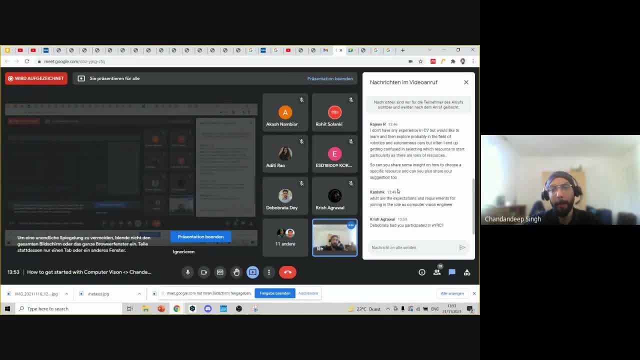 But to start, you should just focus on using Ross for that, for mobile robots, And you can use visual slam packages to actually just make it work. It would be very simple to start with, It would not be very complicated And if you want to go into mobile robots, 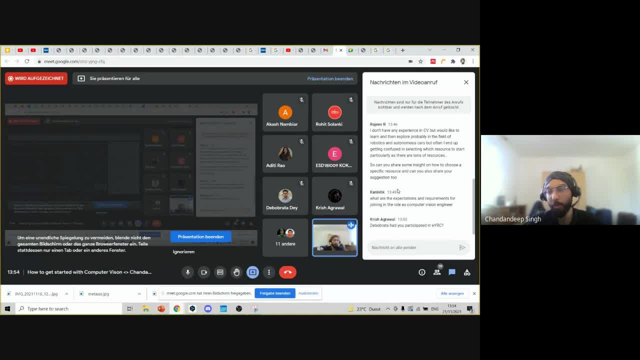 I think, mobile robotics. you would be needing some Ross knowledge as well. So take up a very simple project. let's say visual slam for TurtleBot robot Right, And you can find lots of tutorials online for that. And once you have done that, OK, now you maybe want to take it to another. 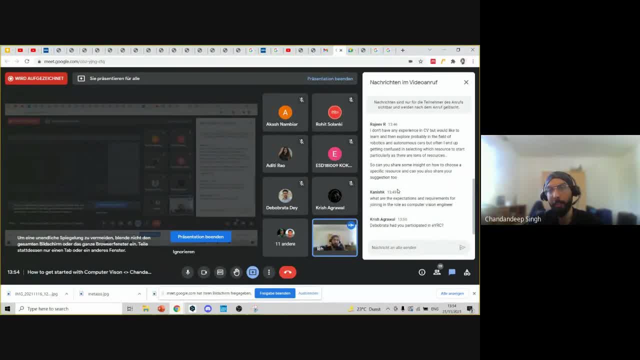 level, so you expand on it, you search what are the different things that you can do: maybe tracking and following the mobile robot, maybe follows some human or something like that, or maybe you buy an actual hardware and do it on that. So that would be the thing. 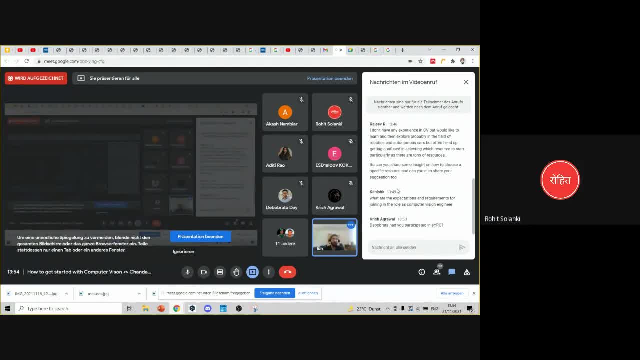 Did I get your question correctly, Rohit? Yeah, you got my question, You are correct. OK, I think Krisha has also raised his hand, but before that I think there were a couple of them who asked in the chat box. could you go through the chat box? 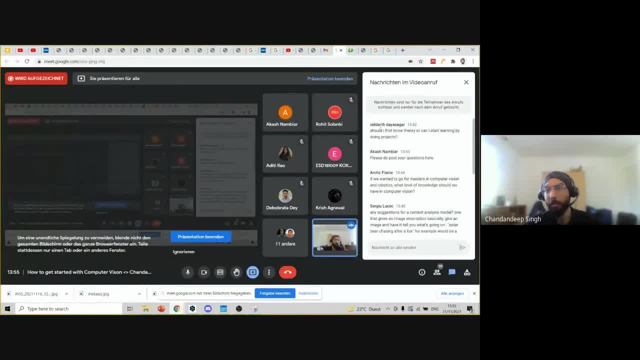 Should I just read it for you? Yeah, sure, I'll go through it. So Siddharth Daya Sagar is the first one, right? Yes, Should I first know theory, or can I start learning by doing projects? This is a very common question, right? 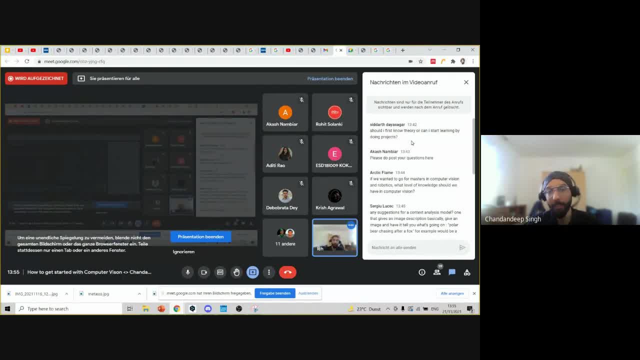 So for me, how I learned was, of course, I was in the university, So I learned theory, theory, theory, And then I did some assignments of all the theory that I did. But for me, what was the best way to learn? 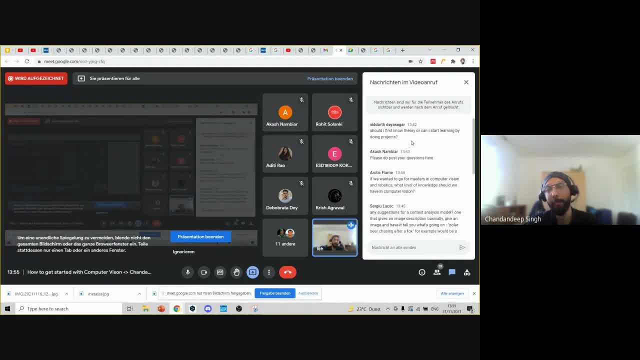 was when I actually got to work in industries and I did projects actually, because of course you know theory and it's good, But eventually if you work for a company you have to have the skills. And I would say, just start doing projects and you can do both of these things. 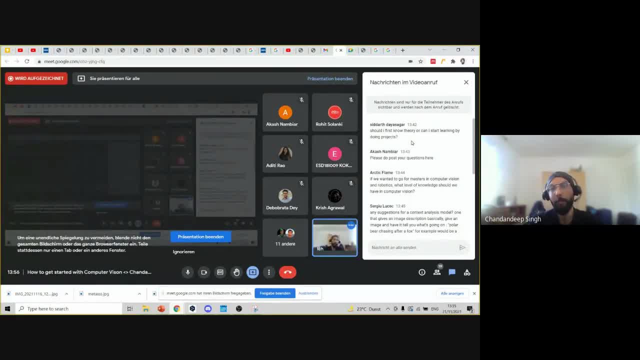 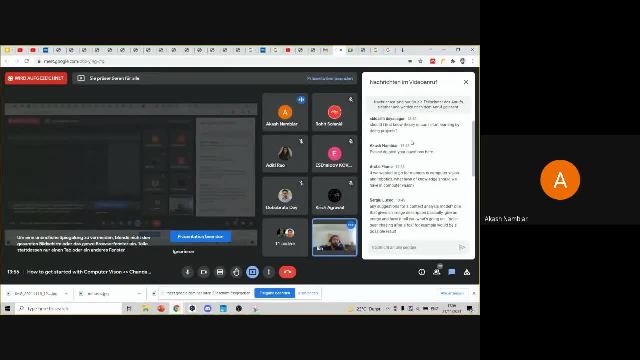 simultaneously. but I would say: focus on projects, And I hope that answers your question. Oh, yeah, So, Chris, you can go ahead. actually, that will go ahead with other questions. Yeah, thank you, So I wanted to know that. 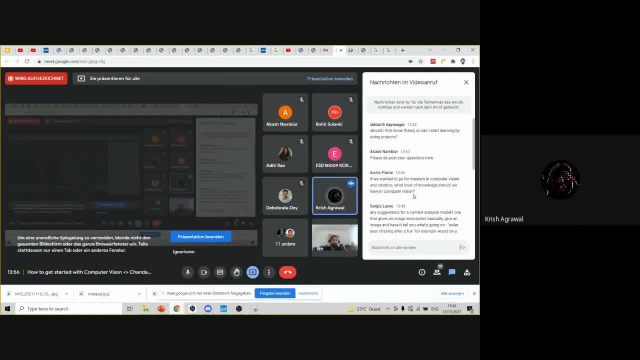 which programming language I do use. to start with computer vision, Yeah, that's also a good question. so it depends on what exactly you're doing, if you're going to be using computer vision for hardware, Let's say robotics or I don't know. 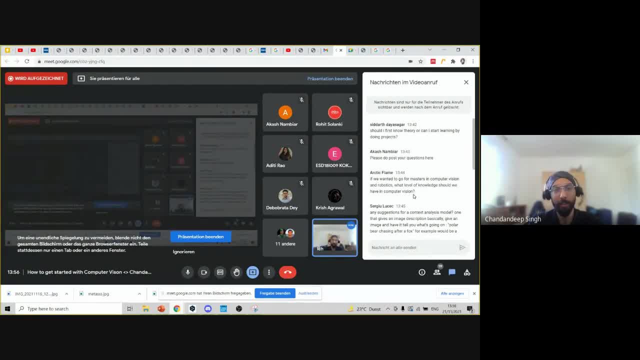 optical instruments or other sort of gadgets. I guess C++ is is more widely used and it would help you. So I think for computer vision C++ is is really a good option, especially when you want to go for advanced projects or or if you want to go for a PhD. 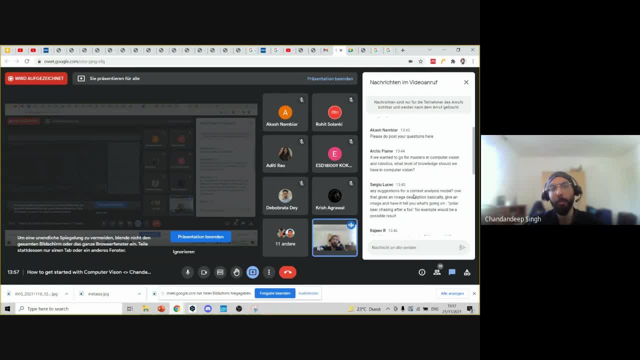 So yeah, this would be my suggestion. But for computer vision, I would recommend that eventually, at some point, you switch to C++ or you also develop some skills in C++. Yeah, thank you, And do you recommend any books by some authors? 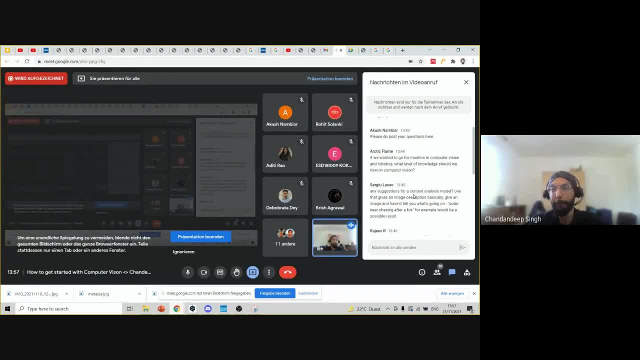 Yeah, the books are standard. So the one is: what was it? The pattern pattern recognition machine learning? I forgot the author name, but I would not. Yeah, I don't. I would not recommend you reading all the theory from the books. 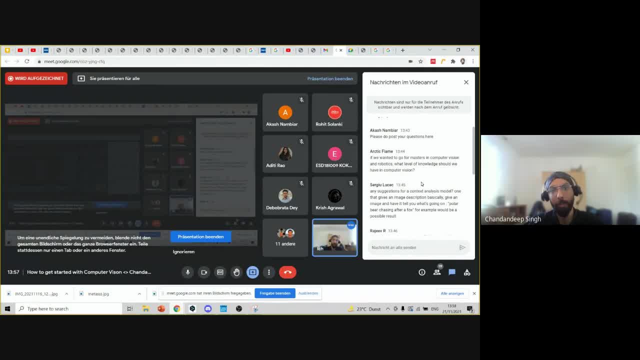 If you can find a book which has lots of Projects and step by step tutorials, I think you can search for that. but apart from that, if you're not going into research, I would not recommend you spending too much time on theory. and use the book. 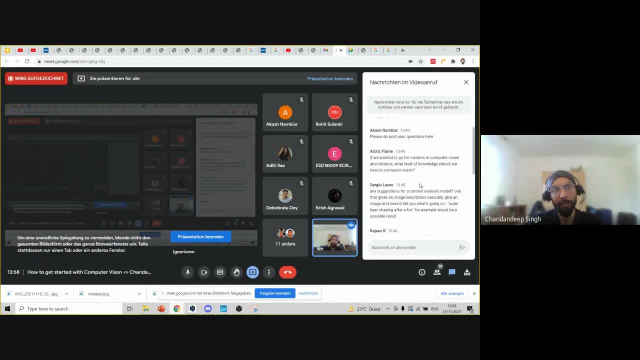 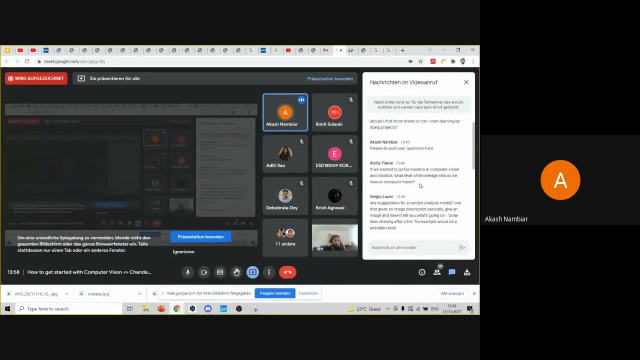 when you get stuck with some of the problems, to see: OK yeah, this is the theoretical concept that I was missing. Thank you, Yeah, thanks, Go ahead. Other questions. we have less time so we'll be closing off soon. 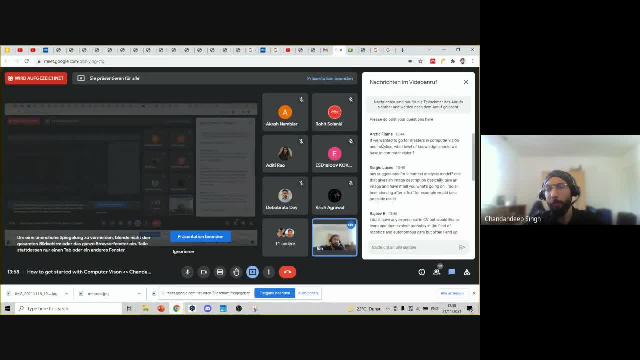 OK, yeah, Yeah. So if we wanted to go for masters in computer vision and robotics, what level of knowledge should we have in computer vision? Well, it, it depends. So I can tell you my journey. So I didn't have any experience in computer vision before I got admission. 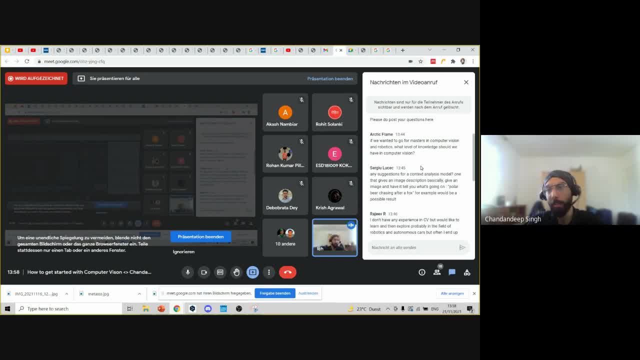 into robotics because, yeah, it was robotics first of all, and not specifically computer vision. So the prerequisite was that I work in something related to the course that I was trying to get admission into, And so I worked in mechanical design, where I worked on some 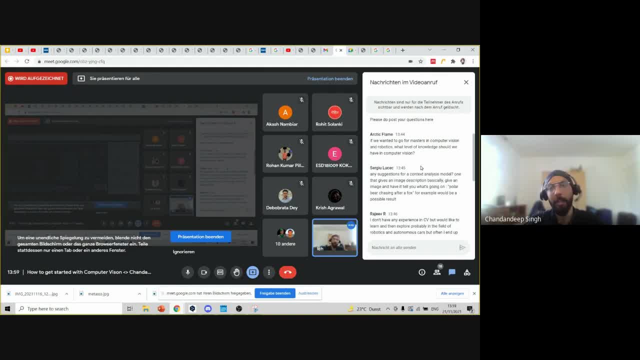 electromechanical mechanisms and other things related to mechanical design And and I did some robotics projects in my college, But I didn't work with computer vision And if you're, let's say, going into robotics, you don't specifically have to have computer vision experience. 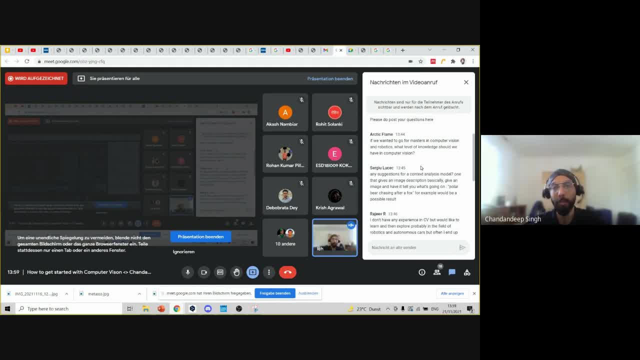 You could have worked in embedded systems and you could- even if you have good profile, I think you can- get an admission in robotics. So because robotics courses are also very interdisciplinary- for example, my course had multi body dynamics, computer vision, machine learning, of course, and but also electrical drives and things from all different fields- 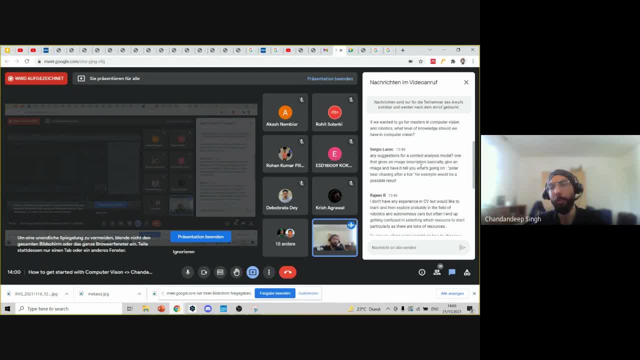 So I would not say that you have to have computer vision, but if you want to, if you want to gain experience- I think Coursera courses or PI image search, you know you can get certification from that- That would be very good quality resource actually. 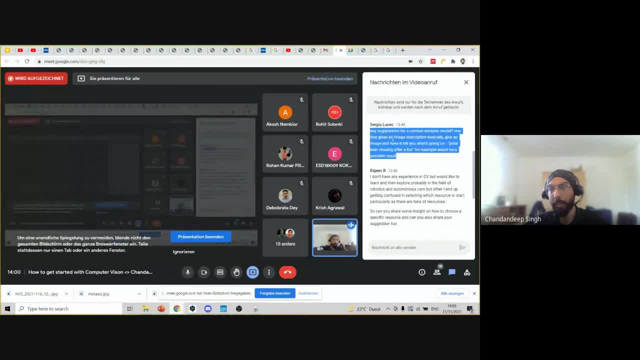 OK, I hope that answered. and the next one is any suggestions for a context analysis model, one that gives an image Description. basically give, basically give an image and have it tell you what is going on: Polar bear chasing after a fox, for example. 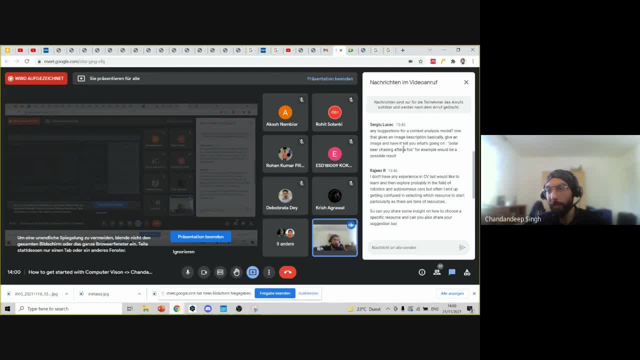 would be a possible result. Yeah, So I have not specifically worked on a project like this, but what would be beneficial is if you go into searching for RNN models, reckoning a recurring neural networks or Even LSTM in that regard, I think, just search for RNN models. 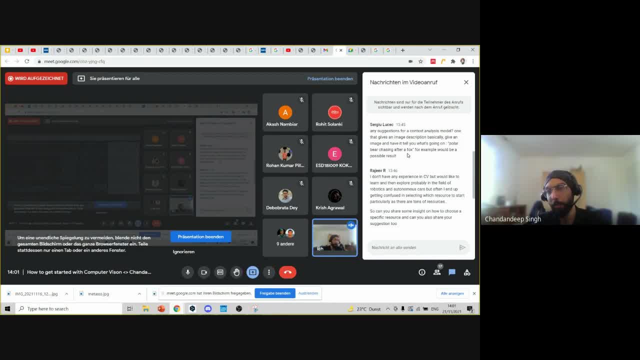 I don't have any specific model suggestion because I have not worked in this. Another one is from Rajiv. I don't have any experience in CV, but would like to learn and then explore, probably in the field of robotics and autonomous cars. But I often end up getting confused in selecting which resource to start. 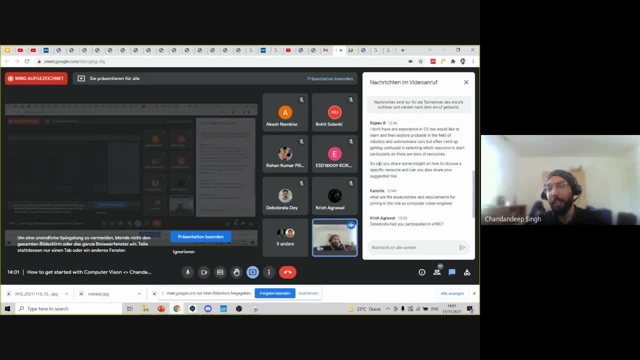 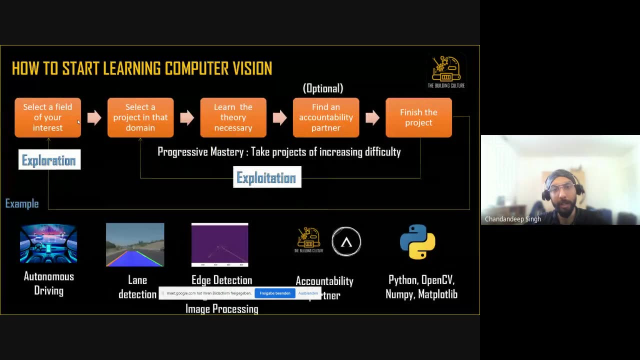 Particularly. Yeah, that's the point Right. So can you share some insights on how to choose a specific resource, and can you also share your suggestions too? So again, the same thing is: don't don't focus too much on selecting the right. 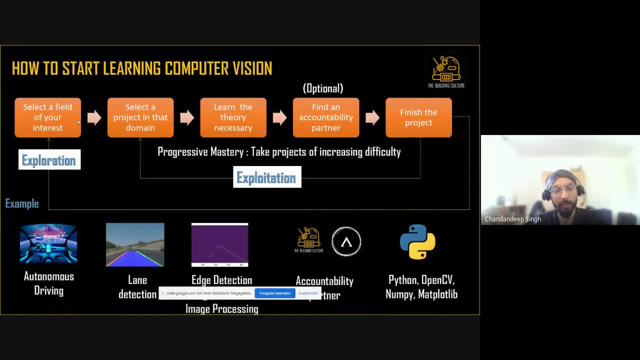 resource, because all of the, I mean if there's a resource from one university and from another university, they would all be most likely very good, Right? So the idea is not to overthink. just pick a project. If you don't like it, leave it right. 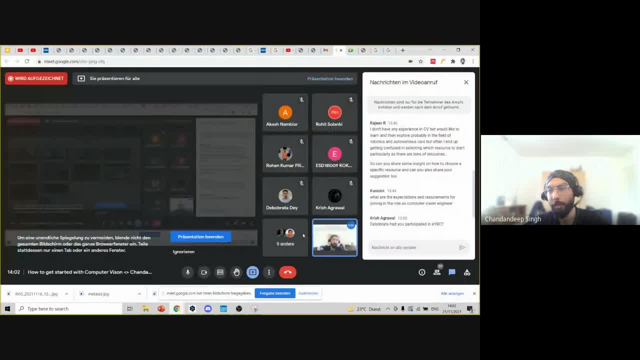 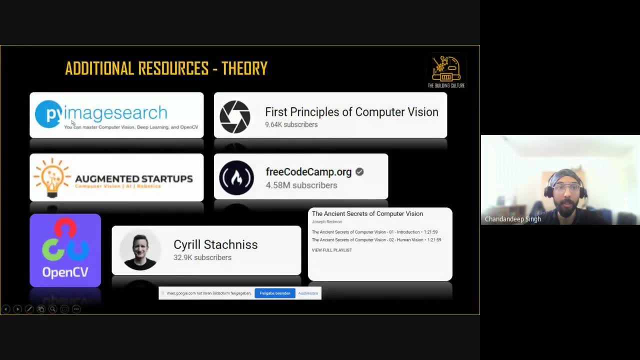 Just try to keep it as hands on as possible, And some of the resources that I can definitely recommend is PyAimit, Search this one particularly because it is exactly a project based learning approach, And also, I think, augmented startups, So you can start with. 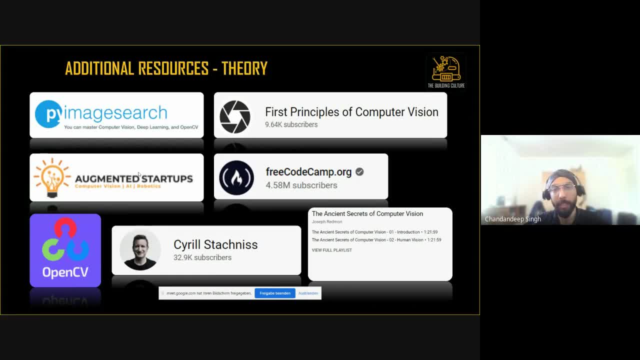 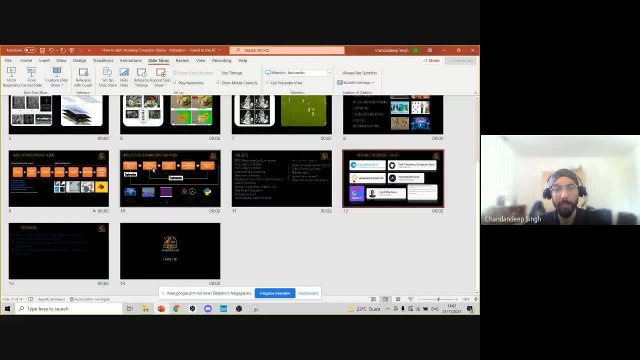 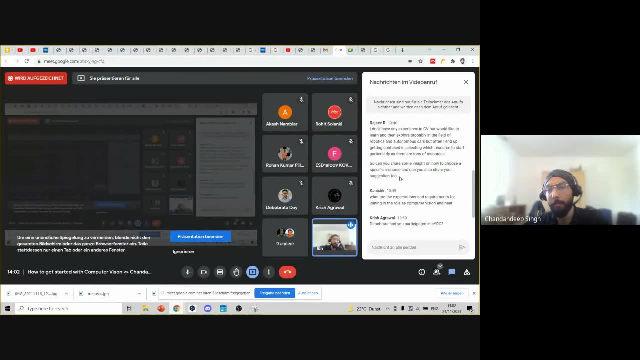 not going into the core mathematics or taking textbooks and reading all of that, but rather taking open CV projects from these tutorials where they guide you step by step how to learn. So can you share some insight on how to choose a specific resource? Yeah, So resource wise, these would be my. 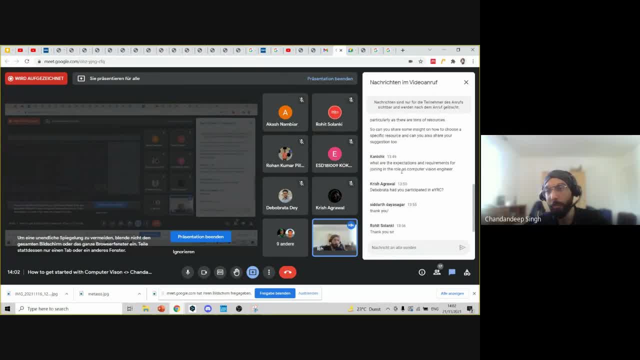 suggestions, but don't think too much about choosing the right resource. What are the expectations and requirements for joining in the role as a computer vision engineer? So, yes, So the requirement would of course be that you have some experience before in computer vision projects. 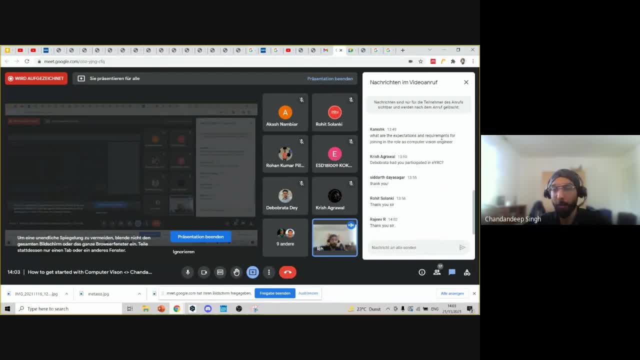 That is the reason why I try to emphasize the importance of doing projects Right, Because once you have the project, build a portfolio, build a GitHub page or just have it organized on your GitHub repository or something, And when you have worked on it, then you 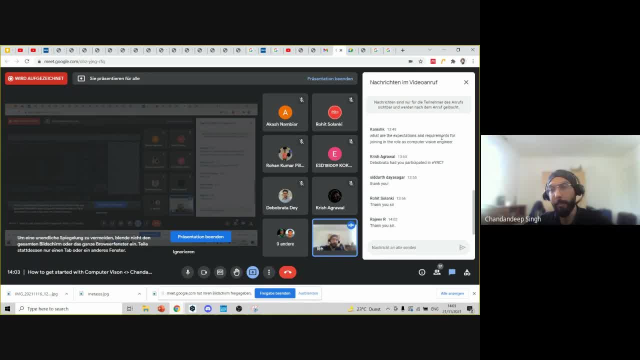 can, of course, explain it to the employer, and taking up additional courses also helps. So compare these two scenarios Right? So one guy who has done computer vision. he has taken all the courses in the university and with excellent grades and everything, maybe also taken some online courses, but he has no projects. 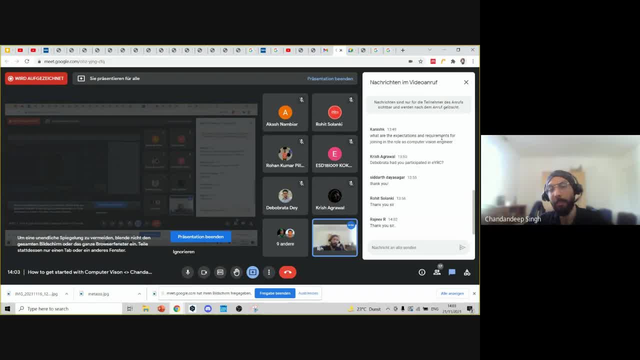 And the other guy whose grades are maybe not that good but he has, let's say, five to six different projects, or even similar projects, but in computer vision. So So yeah, just I think requirement would be to focus on skill development and expectation. 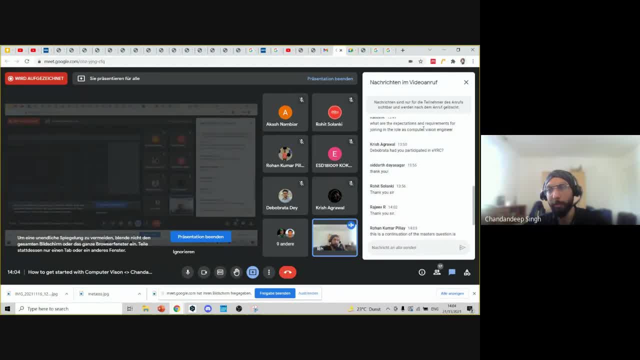 I think expectation you mean after you start working, what to expect. So it depends, I think, on, of course it depends on the company. in a startup You can expect that you would probably be involved in other areas apart from computer vision as well. in a bigger company, 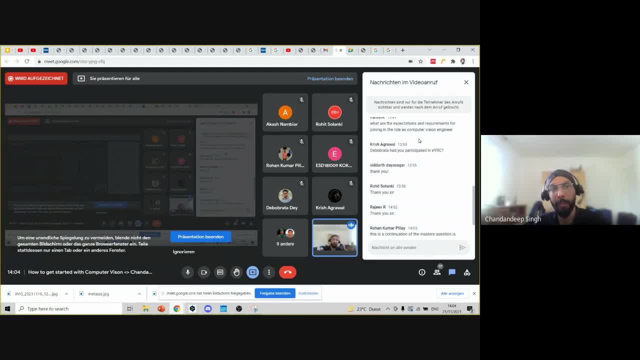 Maybe you will be just focusing on computer vision and maybe in a different role, You can have to focus on something managerial, But also software. So it depends actually, I think that's it right for the questions. So yeah, I think there's one question. 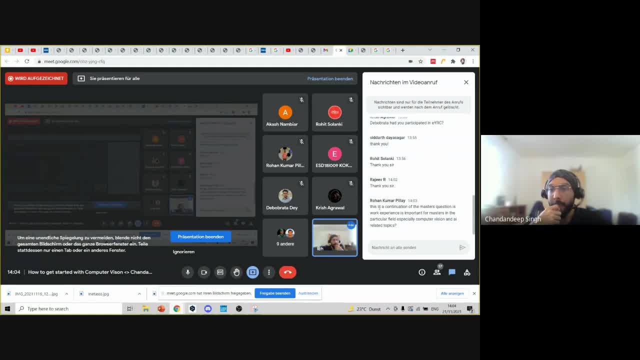 So this is a continuation of the master's question: Is work experience important for masters, in particular field experience, especially computer vision and AI related topics? Yeah, so, as I mentioned, like you don't have to specifically have experience in computer vision to get a master's in in robotics or AI. 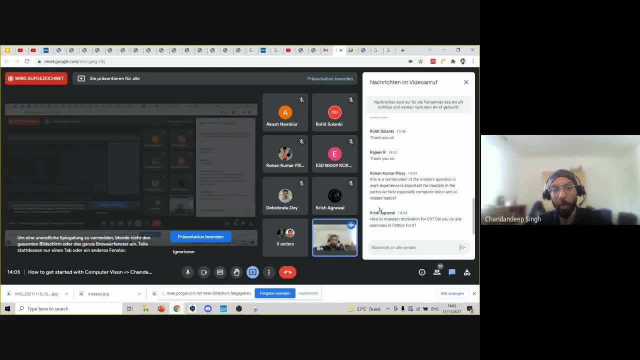 because you're, because they understand that you, you want to study it, And the reason why you want to study it is because you don't know it already, Right? So if you the idea is, you have to demonstrate your motivation and your work ethic, which you can demonstrate by having worked in a, in an R&D, let's say in in a. 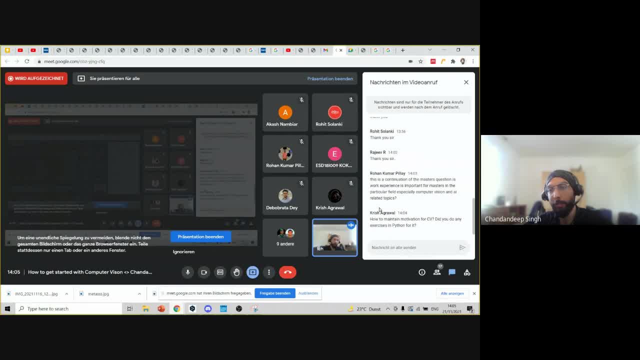 similar area, but it doesn't, I think, have to be specific to computer vision. of course, if it is specific to computer vision, it helps, and it also depends on the university and all. So, yeah, that would be my take. how to maintain motivation for C. 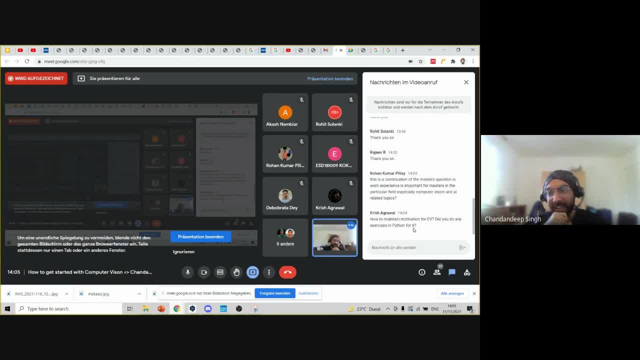 Did you do any exercises in? what do you mean, Chris? How do you maintain motivation for C, Like when you get stuck right? Yeah, I mean it's. it can be hard sometimes because the debugging takes a while And maybe you'll get you're stuck at a problem for several days, but you have. 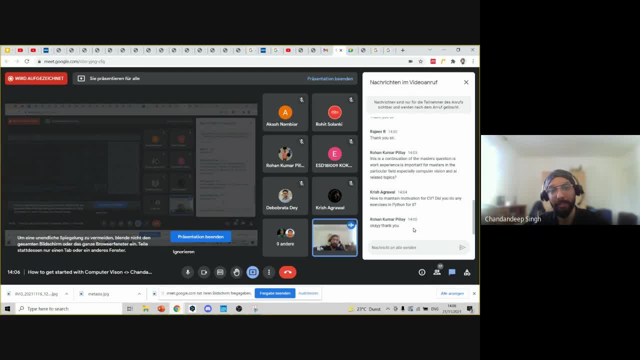 to grind through it and then eventually you will be, you'll get to see the results of your amazing work or whatever you're doing, object detection or whatever. So you know, I think we are all be over our time, You know, yeah. 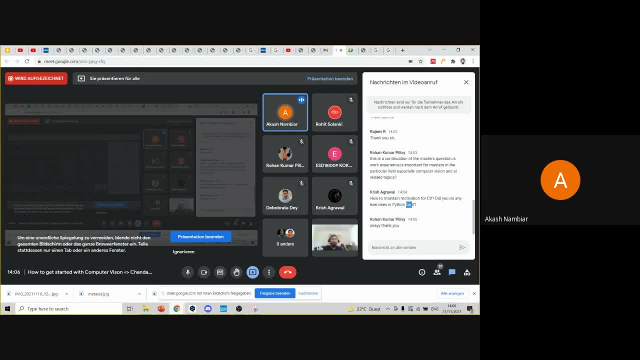 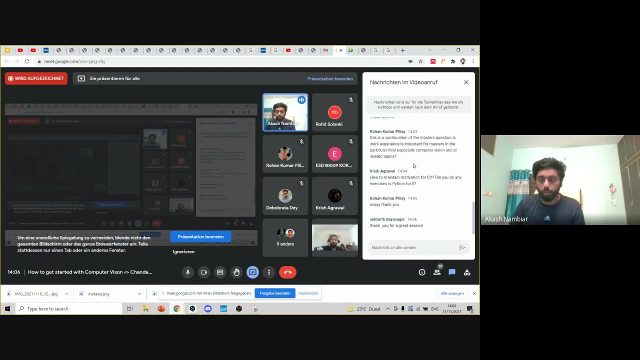 So I think we can stop it and stop the questions here. I'd like to personally thank you for, you know, coming over Our community and doing a session on computer vision, especially getting started, so I hope this has been very useful to people who are joined.